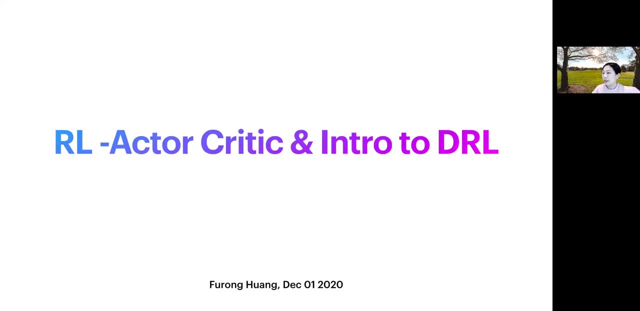 you know some kind of very brief introduction, summarization of the lecture, but it will be asynchronous, So I'll just upload the video sometime for you to review the entire course, but we won't have a formal lecture, You know. so yeah, it was, overall, I think, the lectures for reinforcement learning seems to be. 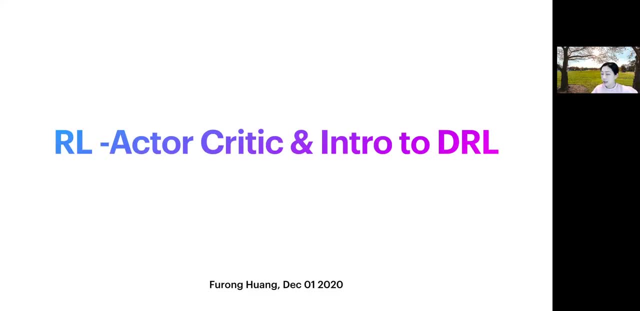 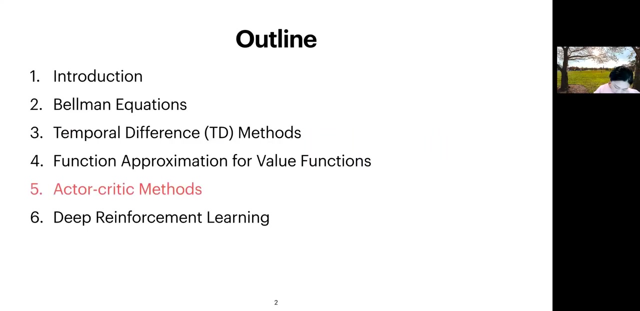 I think people are giving good feedbacks, And so so you know, I guess I wanted to do a summarization of what we've covered so far. So we started with, you know, the introduction RL diagram, and we did talk about the derivation of Bellman equations. I think that's you know. 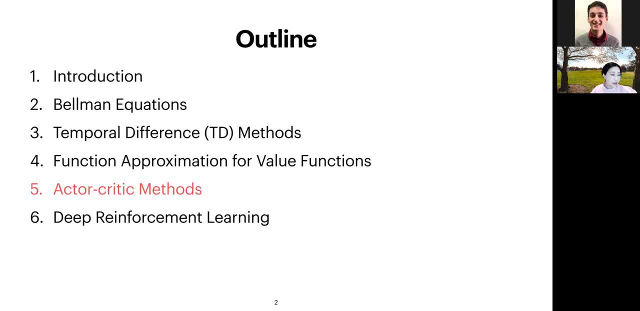 one of the most important concepts, And so we started with temporal difference methods, the TD methods, and it turns out that a lot of the methods that we'll be learning later on are kind of related to TD methods. So then you know, we 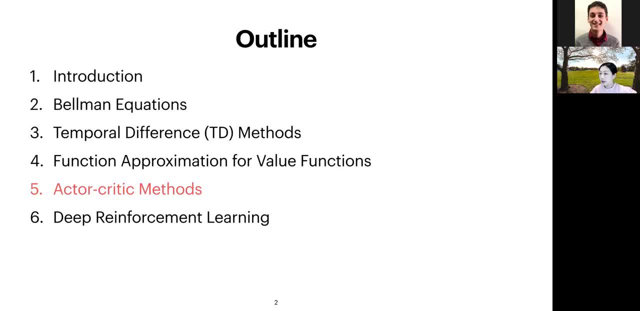 will focus on the more practical scenario. when you have large state space or action space, you want it to do functional approximation for value functions or even for policies. So today we're going to learn something in the middle, or something a combination of the two. 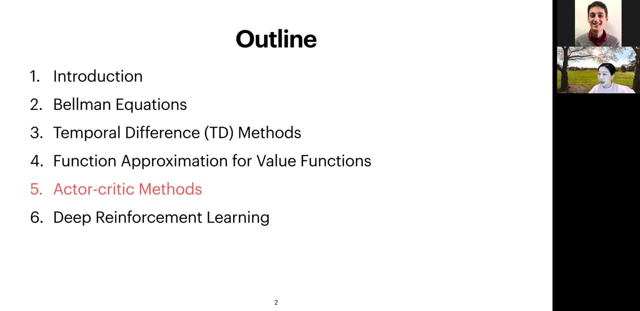 which is so-called the actor critic methods. But overall, hopefully, what we've learned so far would serve as the foundation for learning. you know why some of the deep reinforcement learning methods are doing. you know the things that they're doing, So we'll be talking more about that next lecture. 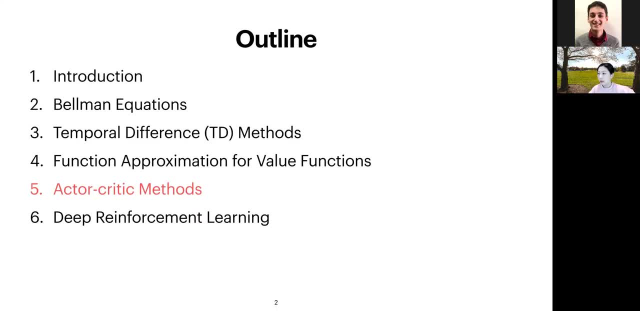 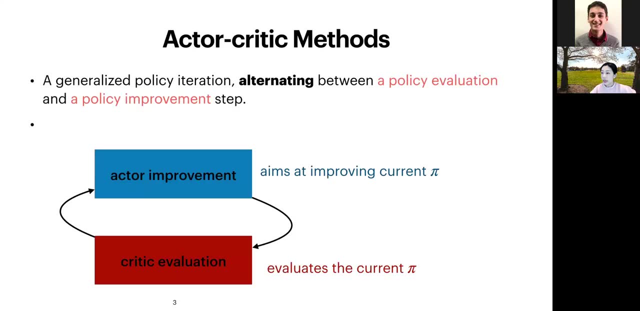 but this lecture will be focusing on actor critic and some introduction to deep reinforcement learning. Okay, so actor critic is actually a meta-algorithm. It's so-called an actor-oriented algorithm that is used to evaluate policy changes, So it's a kind of a general policy iteration. We talked about policy iteration very briefly. 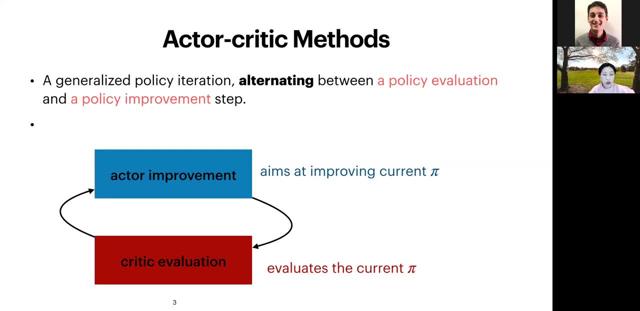 when we introduced, you know, reinforcement learning. So it's alternating between a policy evaluation and a policy improvement step. So you know, you can see, here I have this blue box and the red box. Blue box is actor improvement, right? So this is the. 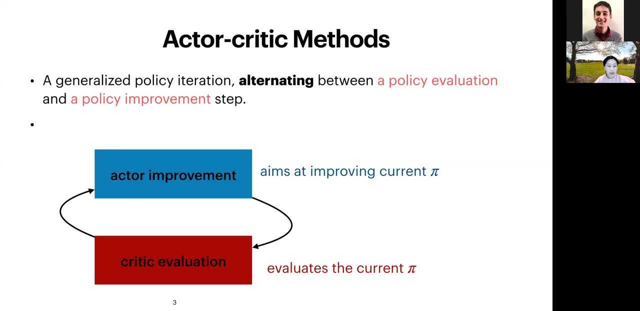 critic evaluation. So the actor aims at improving current pi by getting the information output from a critic evaluation, usually a Q function evaluation, And then the critic, you know, by receiving a pi, could evaluate, you know, the value of the pi or the Q of the pi right. 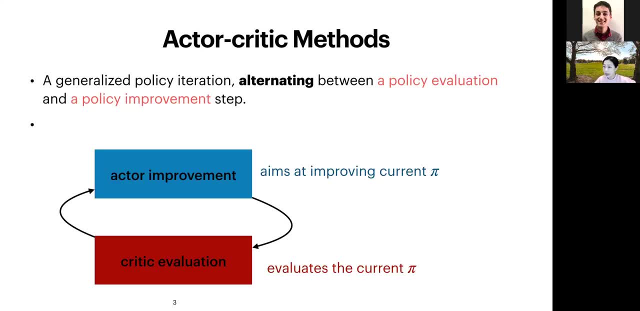 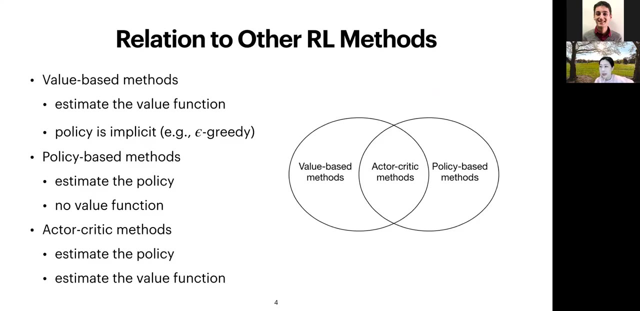 So that's, you know how they are collaborating And essentially this, you know you can do this iteratively. That's why it's called a policy iteration. It's also called a generalized policy iteration. So you know, I said it's kind of a combination between the 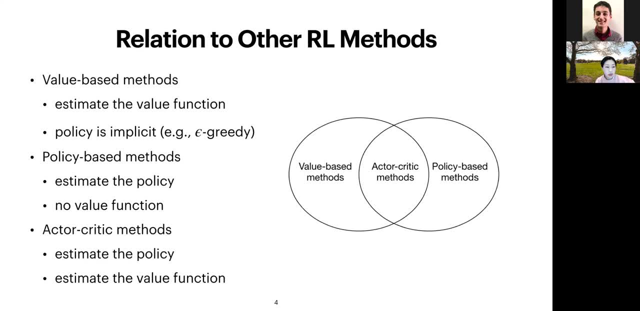 value-based methods and the policy-based methods. So you know, think about this. What's a value-based method? Basically you can estimate the value function right And you know policy is kind of implicit. We don't explicitly work on improving the policy. You know we often for 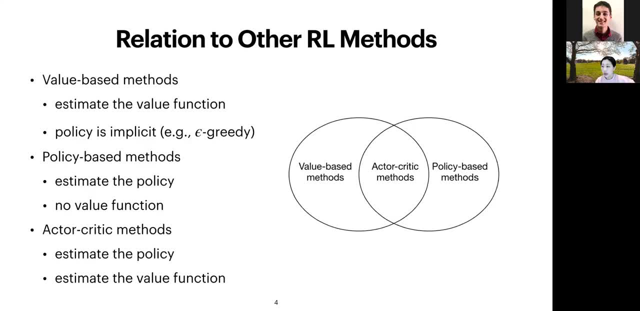 example. you know we learned about Q-learning. Actually, I guess you know CELSA may be a better example. CELSA kind of implemented an epsilon-grady kind of algorithm, right. So epsilon-grady policy, So that's value-based methods. But what about the policy-based methods? So policy-based methods. 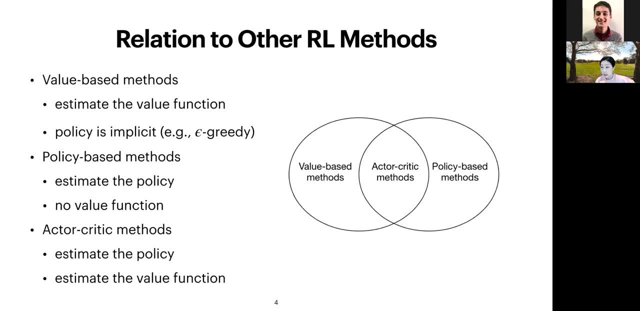 essentially estimate the policy. right, It is explicitly working on the policy And you know, of course, there is no value function explicitly evolved, right? So you know, only the policy is kind of explicitly evolved And you know we're working on improving it. 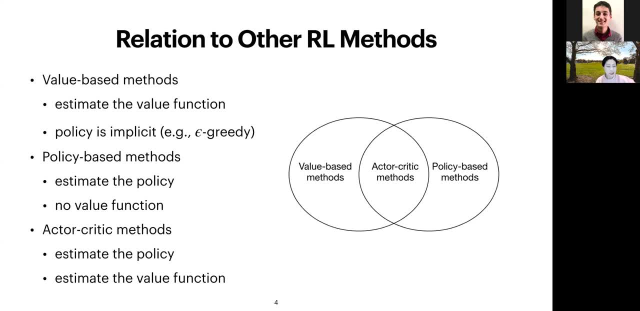 So the actor-critic is the combination of the two. It is estimating the policy, but it's also estimating the value function, So it is explicitly working on both. So that's you know, probably the reason why sometimes actor-critic methods work very well. 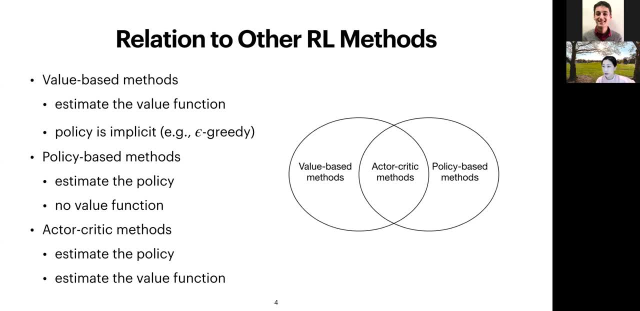 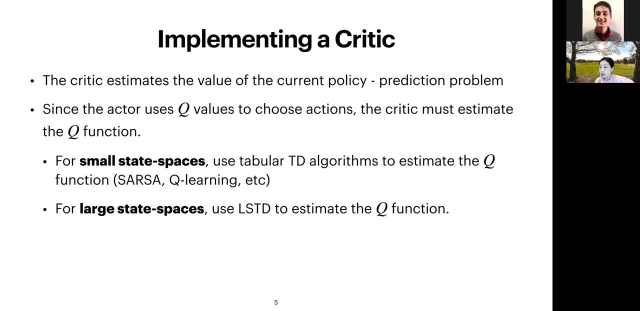 You can see the diagram on the right-hand side here, right, So you can see the overlap between value-based and policy-based and essentially it's the actor-critic methods. So you know, we talked about this as a meta-algorithm, right? So it's like a generalized policy situation. 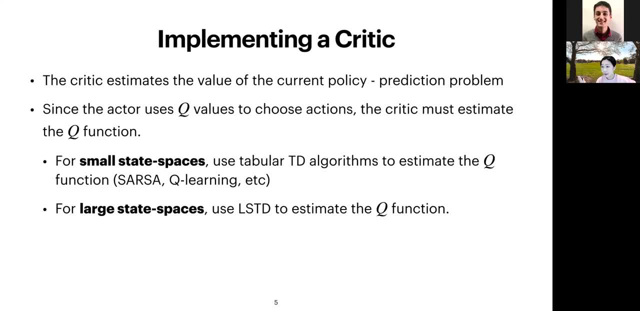 but it's a meta-algorithm. So the question is, how do you implement a critic? So the critic implementation basically estimates the value of the current policy. So it's a prediction problem. you know, if you wanted to use the machine learning language terminology. 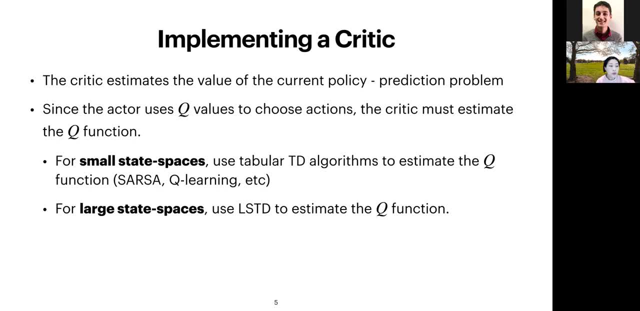 to describe it. It's really a prediction problem. So the actor is going to use the Q values right? Where do you get the Q values, The critic right? So here it's saying that the actor will have to use the Q values to choose actions and therefore the critic evaluation. 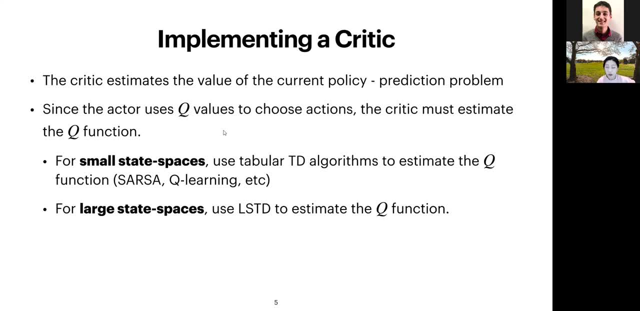 is going to do that. The critic must estimate the Q function. So here I'm just listing a few different scenarios for smaller state-space and the large state-space- Again not talking about a specific algorithm here, but I wanted to frame it as a meta-algorithm, right? So for the critic, 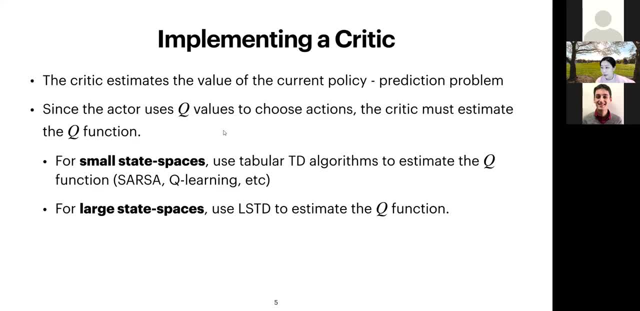 if you have small state-space, then of course you know it is tabular, So you can use tabular TD methods, right, For example. we'll learn. you know, if you have a small state-space, then of course you know it is tabular, So you can use tabular TD methods, right, For example. we'll learn. 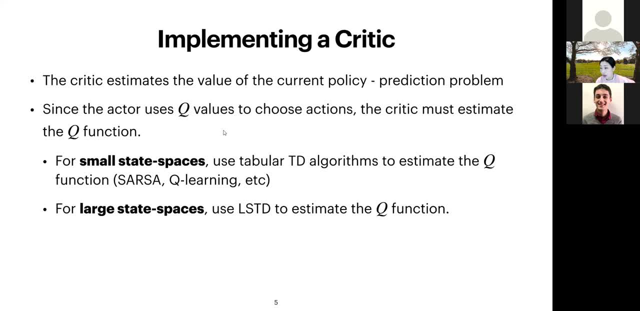 about SELSA. we'll learn about Q-learning, we'll learn about expected SELSA and so on. right, So you know what we've learned so far could be used in this critic when you have small state-space, okay, But also we learned about- you know, function approximation, right. So when you 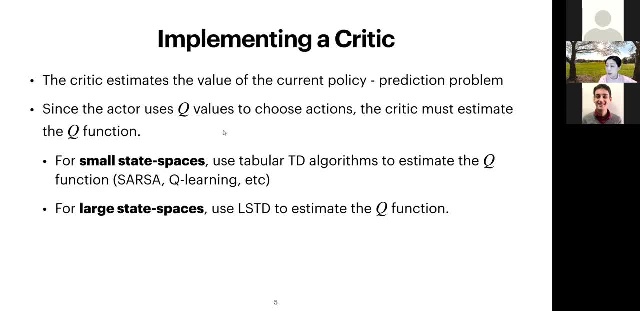 have large state-space. So again for large state-space, you could again use what we've learned so far, like you know, LSTD, For instance, to estimate the Q functions. So if you go, so if you go back to the next, 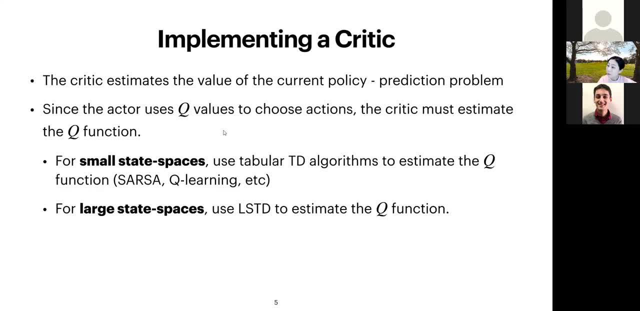 the previous lecture, you will notice that we learned about value-based methods and policy-based methods. So these value-based methods for function approximation could be used here. okay, And of course I'm just using the example here. So let me see in the chat. 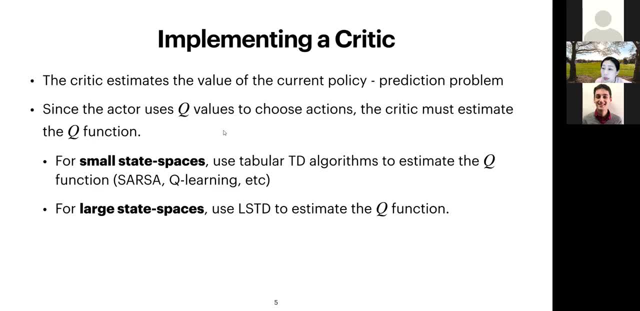 state-space is small, but action-space can be large, so it can be infeasible. So is this a question or what is this comment for? Oh, okay, So my question is: in the first case, we are considering small state-spaces. 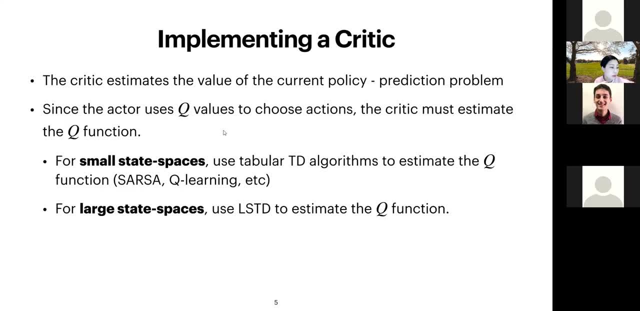 and create some tabular form, like: have the critic in the tabular form, But the but in case the action-space is large, it will be infeasible to create the table also, right, Yeah, then that's not a tabular case, right? 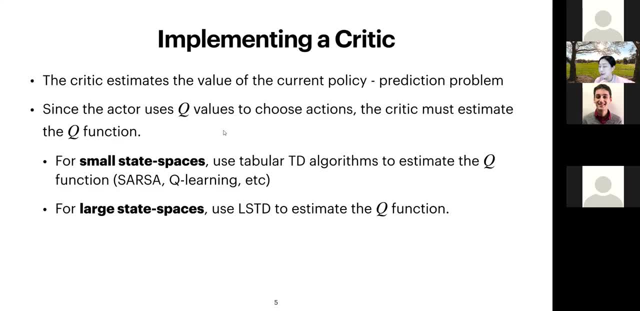 Okay, Yeah, so tabular case, usually you will say you can enumerate the state-action pairs. Okay, okay, Yeah, okay, That's a good question. Okay, so this is what I wanted to talk about in terms of the critic. Okay. 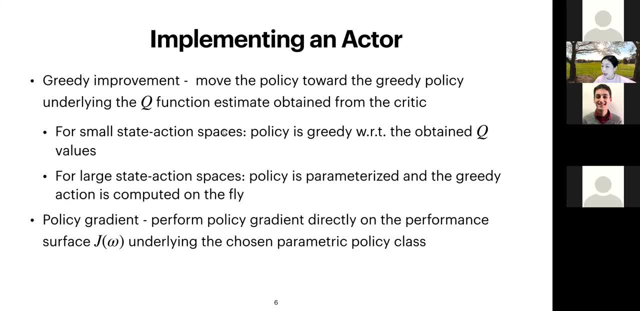 So now you know you might ask: how do we implement an actor, So after? so usually you can do some kind of grady improvement. of course, you know I believe there are other algorithms that are not always grady, So you can move the policy towards the 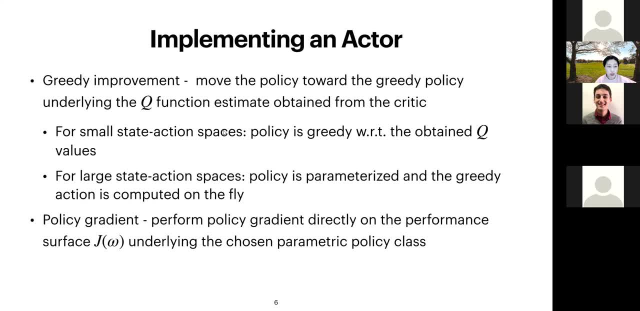 grady policy underlying the cube function estimate obtained from the critic. For example, if you have small state-action pairs um action spaces, then you know you can just have policy gradient with respect to the obtained cube value. so arc max again of the cube right, so for large state action space. so because you 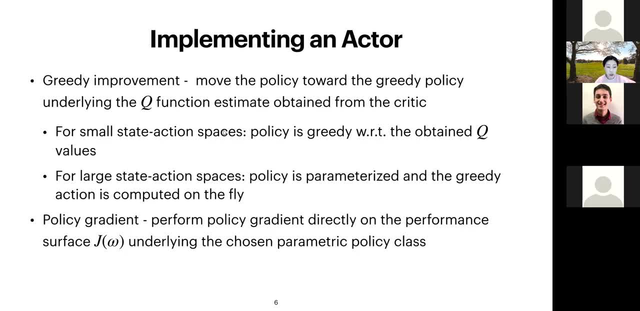 have to do, you know, uh, function approximation, so your policy is parameterized. so then the greedy action is computed on the fly because you have a parameterized form. therefore, you can, you know, just compute the gradient policy based on the current destination of the parameter. okay, right, so this is the gradient improvement. well, in terms of the policy gradient. 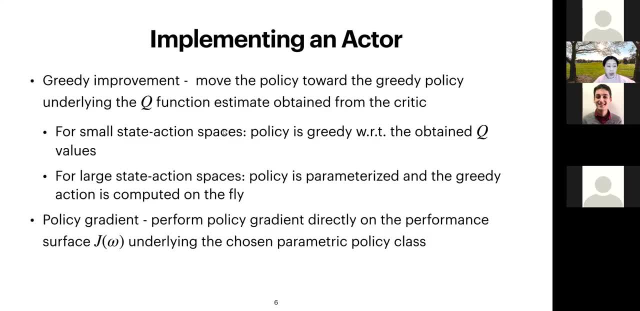 so you know, as we learned before it performed policy gradient directly on the performance surface. you know some kind of uh measure, j omega, right. so j omega sometimes could just be the value uh underlying the chosen parameter policy class. so actually here i wanted to introduce one important um i guess you know- uh modification to the policy gradient we've learned so far. 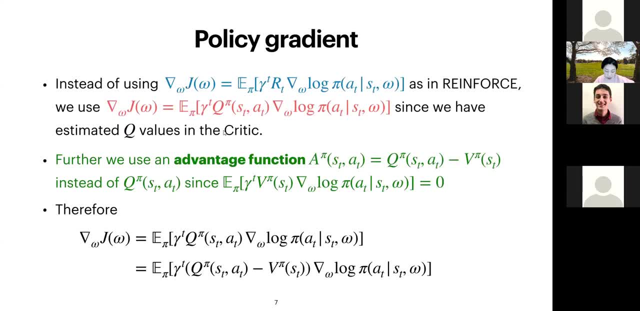 remember we learned about reinforce, um, so in reinforce, right. so, uh, what you do is, you know this here i marked as blue. so you take the gradient of the uh, j, omega, the objective function, right. so? and it turns out, if you do reinforce, then you would actually calculate the gradient as the expectation of the gamma, t, rt, rt is the return. 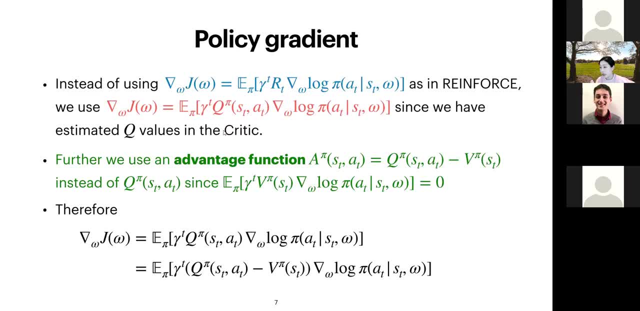 gamma. t is the t's or um power t of the uh discount vector and then the del. you know the gradient with respect to om. logarithm of the pi. okay, so this is what we learned about to reinforce and i kind of talked about why it is the logarithm of the gradient, uh sorry, the gradient of the. 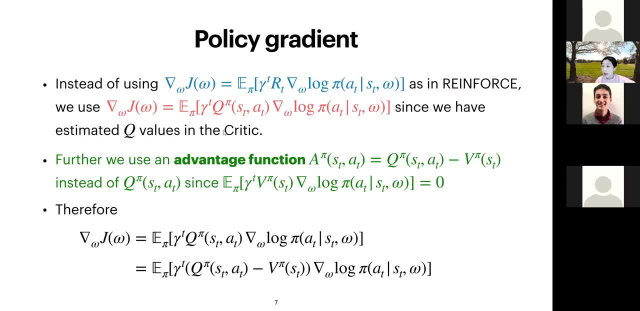 logarithm. so that's reinforced. but a modification of that is, instead of using- uh, you know the return, what we can do is now in actor critic, since we know the value we could use, since we we have an estimation of the q functions, we can replace the return by the q function. 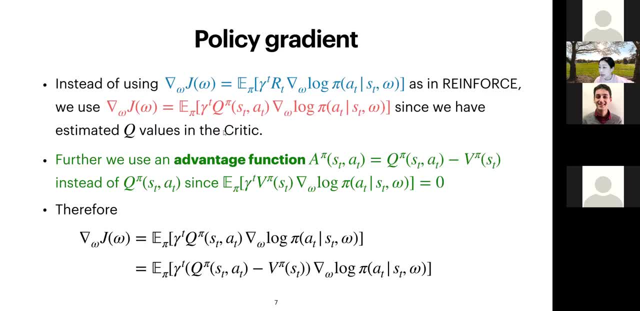 okay, so, so in. so now you know, the gradient estimation is not the gamma, you know power, t, rt and the gradient of the logarithm, pi, but instead is the gamma, t, q, pi of s, t, a, t. okay, so this is a replacement of the return. why, before we don't have the you know q function. 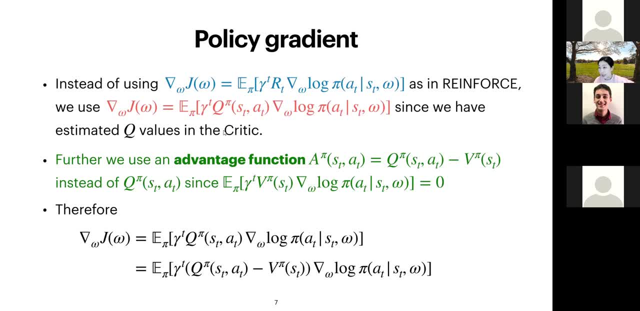 because we are doing a policy gradient and we said that policy gradet do not explicitly work with the q function. but now in the actual critic scenario, we can, because we have a critic that is evaluating the q for us. so we can just replace the r? t, the return, with the q pi s t. 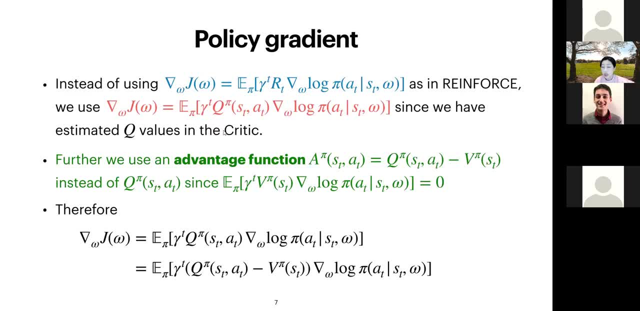 a t. okay, so, um, i guess you know this is not very difficult to answer for you guys, but we got a bit much differentseniorization in the application of q to the q pi, which is the, the creating of the e, the exact same equation for negative and liberals like e- to the q area now. so let's discuss the q function. 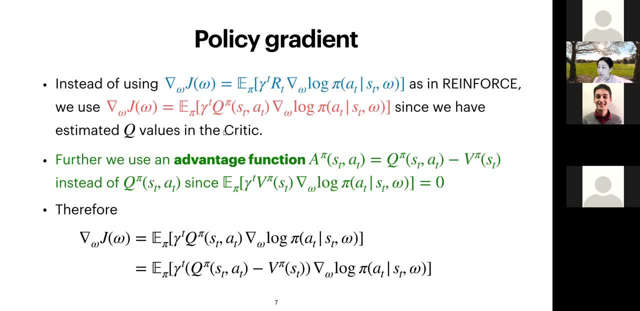 doing a policy gradient and we said that policy gradient e to the q function is not explicitly work with the q function sources. but we set this also because we do not explicitly work with the q function now in the work with the q functions, but understand then more importantly, um, you know, many of you might have heard about the advantage. 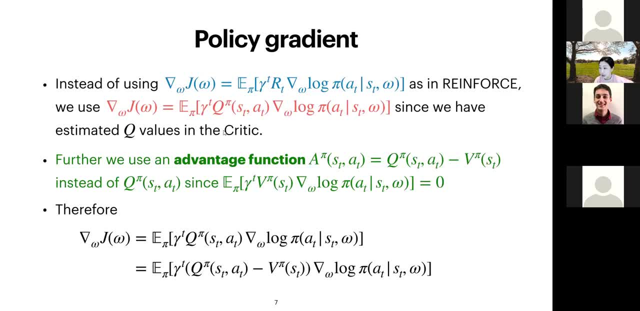 function. but this is a very, very important method for reducing variance. you know, we know that the high variance is indeed a, you know, very serious problem in reinforcement learning. so one further modification to reinforce in this actual critic is to have this so called advantage function. so what is advantage function? 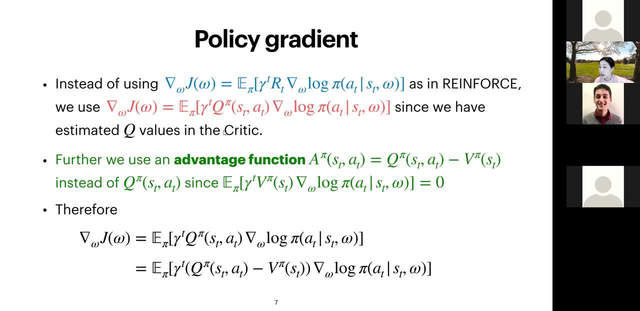 advantage function is the difference between the q and the v. so see, here is the thing. so, first of all, advantage function should be a function, should be a function dependent on s to the state right, because i'm going to for different states, the advantage function will be different. 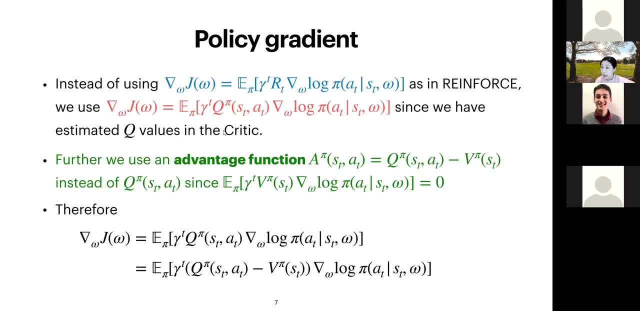 but, more importantly, advantage function should be a function. More importantly, advantage function is a function of the action. So what is the action? So, no matter what the action is, the advantage function is saying if I take that action, how much I can improve by taking that action. 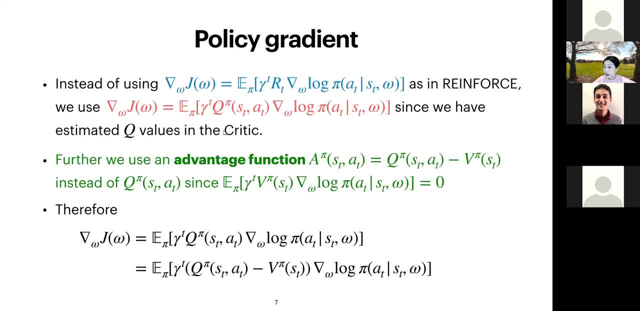 then following pi. so the difference between the value I don't know. Let me say that again. So the advantage I could hope to improve my value function by taking action at at state st, compared with following pi at state st. Does this make sense? 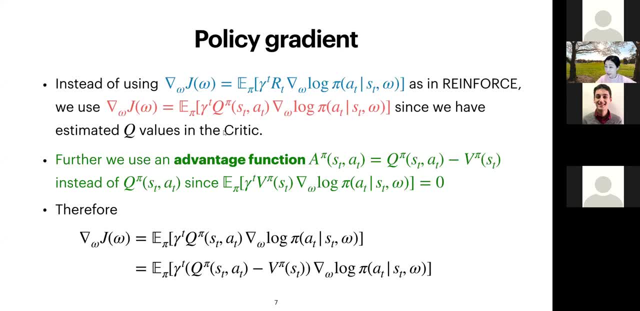 Okay, yeah, so this. so you know why it's called advantage function. It is basically saying I wanted to take action t instead of following pi and I might get an improvement. Definitive advantage function can be negative, right. 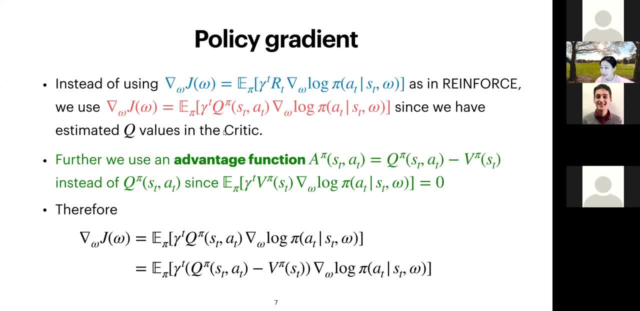 If you're taking the bad action. of course you know it could be worse than the value following pi, But anyway. so we are looking at an advantage function instead of a Q function. Why You know? basically, they're saying you can replace the Q. 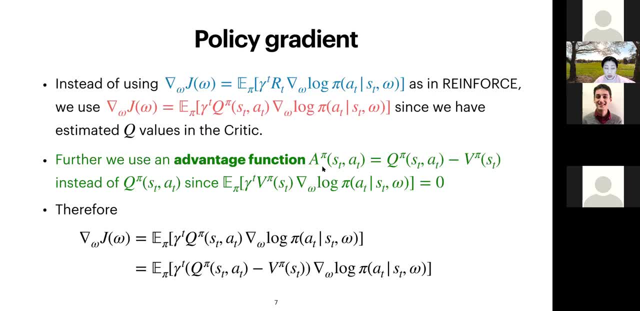 with the A with advantage function. why? The reason is that this part you know, so you know, if you replace that advantage function, you would have an extra return, which is the gamma, t, v, pi, st and gradient of the logarithm of pi right. 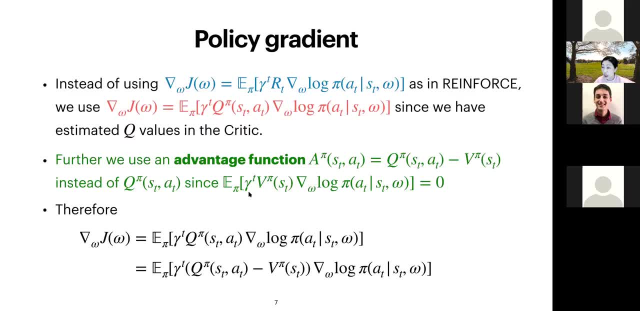 So the good thing about that is the expectation is actually zero, Therefore optimizing, oh sorry. So the good thing about that is the expectation is actually zero, Therefore optimizing, oh sorry, Therefore optimizing, oh sorry. You know having the update function. 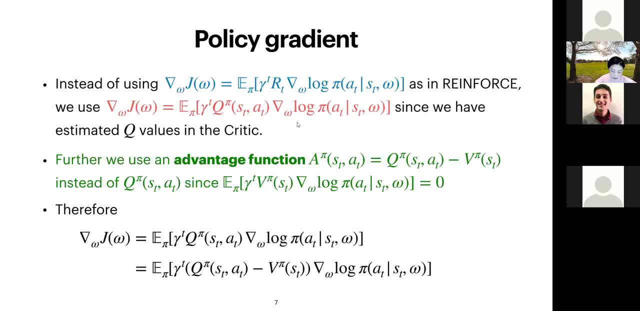 using the red turn. So I don't know if you can see my screen. So you know, doing the update using the gradient estimate. using the red turn is the same as this term here And because this term is actually zero in expectation. 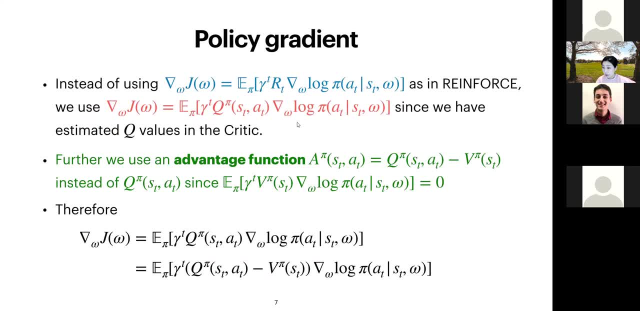 So this is why you know we use advantage function. physically, it has a meaning. It's telling me how much improvement in terms of value I can expect by taking action A. However, mathematically you can prove that by using: 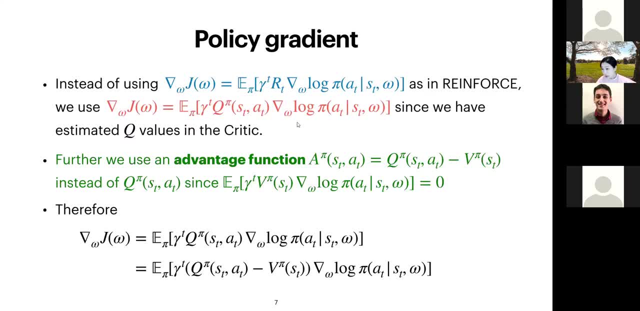 advantage function, you can reduce variance and then the methods will be more robust. Okay, So this is, you know, a very important- I guess you know- technique that people use a lot in reinforcement learning, using advantage function and using the fact that the expectation 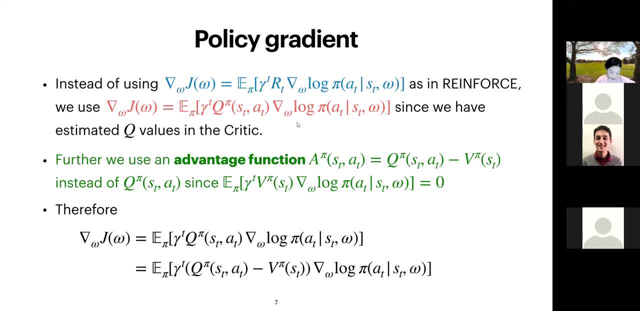 of the value, function and the grade. and so you know, using this fact, can you see my laser pointer? Using this fact? Yeah, And this expectation zero is very important. Okay, Yes, advantage function: basically is a variance reduction trick. 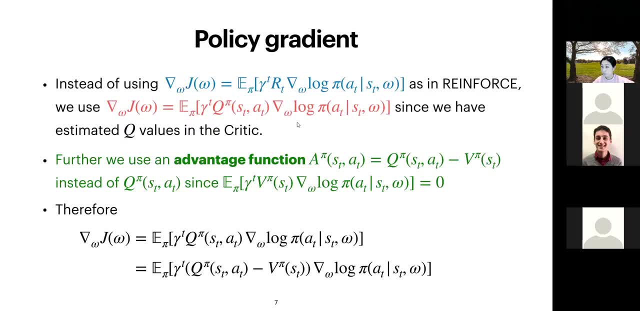 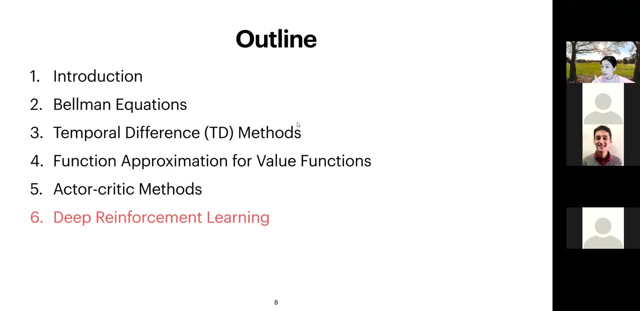 Okay, Okay, Okay, Okay, Okay, Okay. All right, so shall we continue. Okay, so this is the actor critic, right? So, actor critic. really, I don't want you to spend a lot of time on it, because it's really just something. 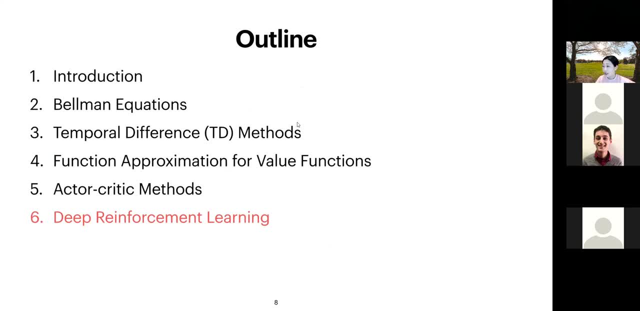 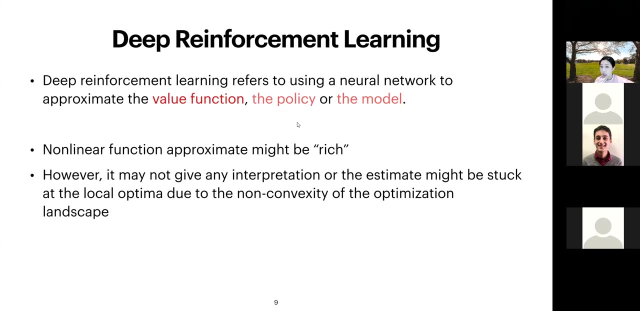 a combination of the value-based and the policy-based methods. you know using both. So now, as promised, we're finally at the deep reinforcement learning. So what is deep reinforcement learning? I guess you know. deep reinforcement learning really refers to using a neural network. 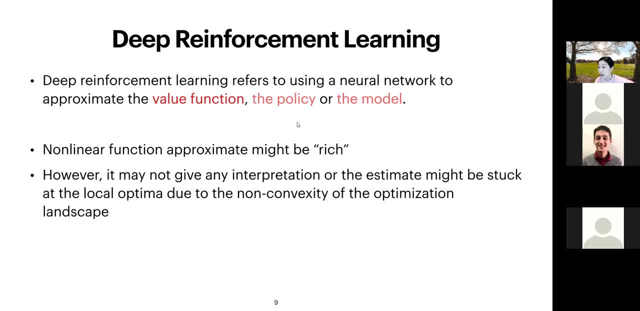 to approximate the value function or the policy or the model right. So you know, we talked a lot about value-based methods and policy-based methods. We kind of, at the beginning of the reinforcement learning introduction to reinforcement learning, we said: you know, we have this transition model right. 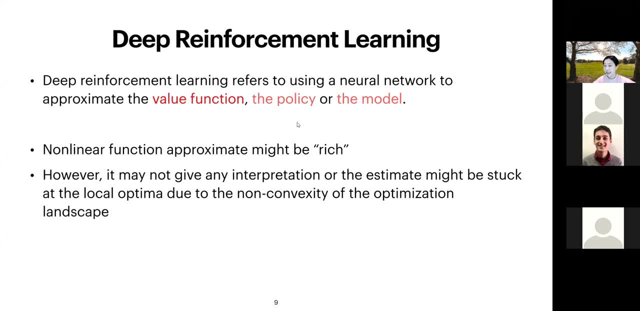 So, but we didn't spend a lot of time talking how you know we can do dynamic programming when we know the model. but I kind of, you know, hinted that you know, if you know the transition model, then everything becomes really simple. 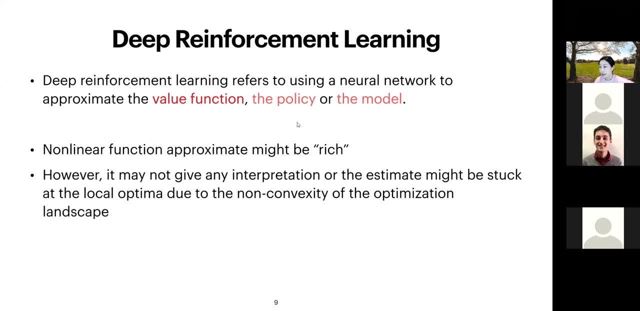 You can just solve dynamic programming and you will get the solution for reinforcement learning. So deep reinforcement learning, it's really just a special way of doing function approximation- either approximation of the value function or the policy or the model- right When I say the model? 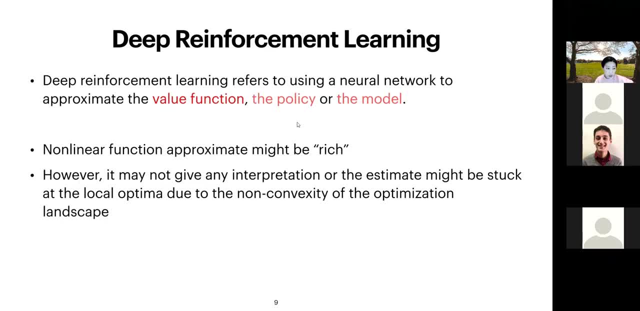 it really means the transition model of the RL. And so you know now, you know, since you guys are familiar with, you know, deep learning. well, you know, instead of using simple function class, hypothesis class, you're using this complex. you know. 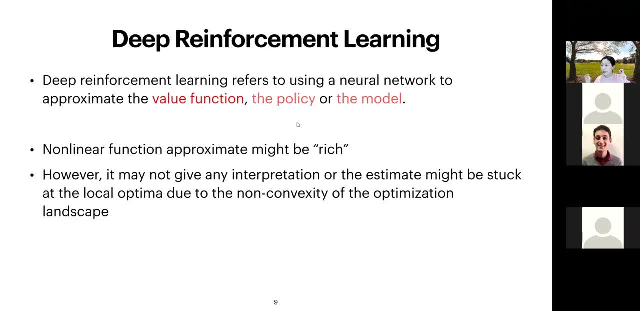 example, they try to solve nonlinear functions. So it's supposed to be a rich right, Supposed to have very high expressive power. And the you know theoretical, theoretical work have shown, you know, the universe of Rosameter kind of theorem. 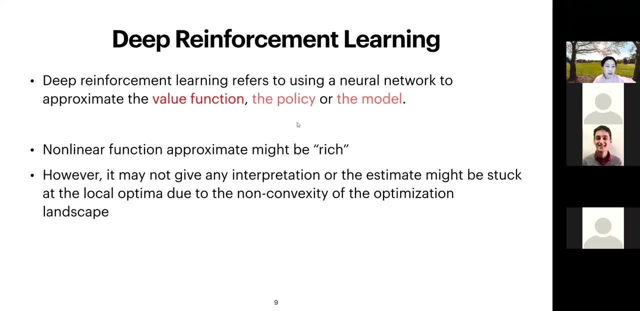 about neural nets Right. So one thing you know: deep reinforcement learning, although very powerful, but it may not give an interpretation right. It may not, or the estimate might be stuck at local optimal, just like we would suffer similar problems. 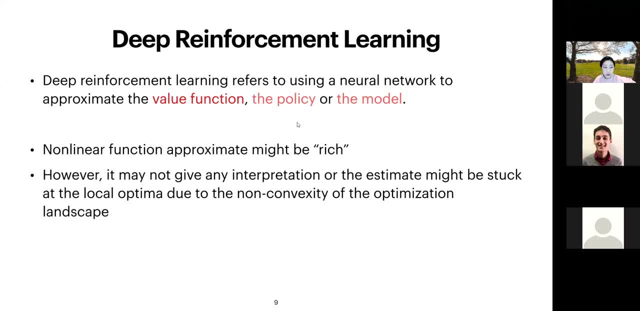 in learning, in traditional deep learning, right. So because we have this non-convexity of the optimization landscape, so indeed we don't know very well about how you can converge to a global optimal. but there were also a lot of work recently. 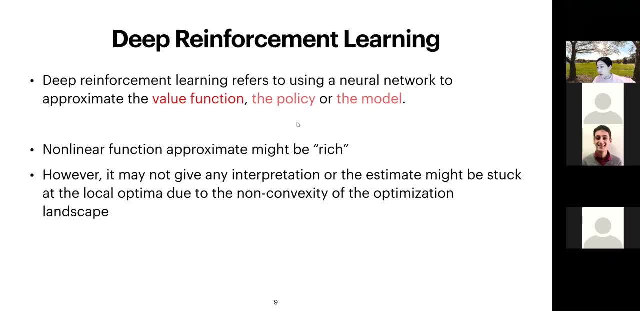 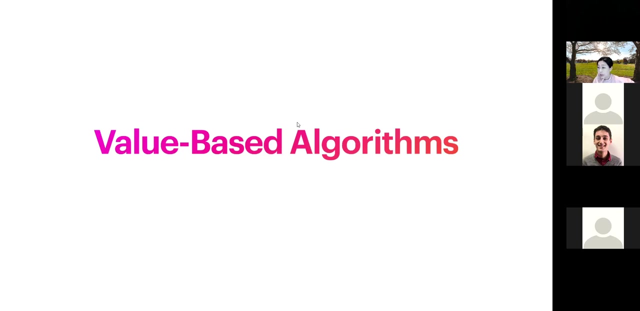 working on understanding the behavior of first-order methods, second-order methods on deep learning, specific deep learning optimization, landscape right, Such as skip connection and things like that. But that's not the scope of the discussion for today, So I wanted to first introduce the value-based algorithms. 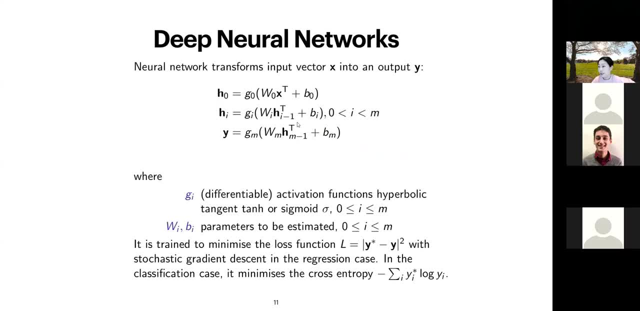 since I'm sure a lot of you have heard about deep Q-networks, So first let me just very, very briefly review the deep neural networks. I mean. so this is just: you have neural network transforms input vector X into an output Y. 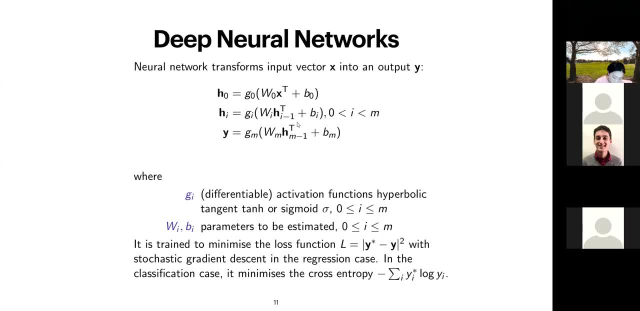 And so you have W zero, X transpose, okay. So you know, you have the input, you have a linear transformation, you have a like a shift term, and then you have a non-linear transformation, so-called activation function. right, 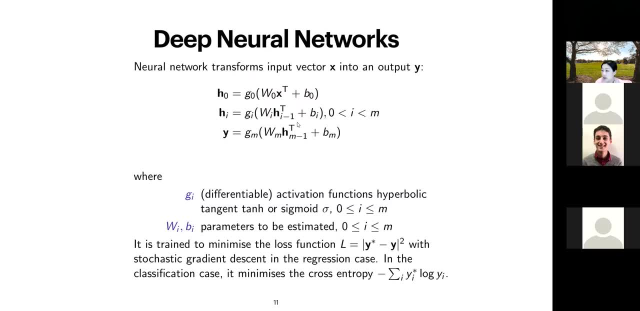 Reload function, hyperbolic, tangent, sigmoid and so on, Group sort and these kind of more advanced activation functions. So once you have that, then you go through. you know, go through another linear transformation, have a shift term. 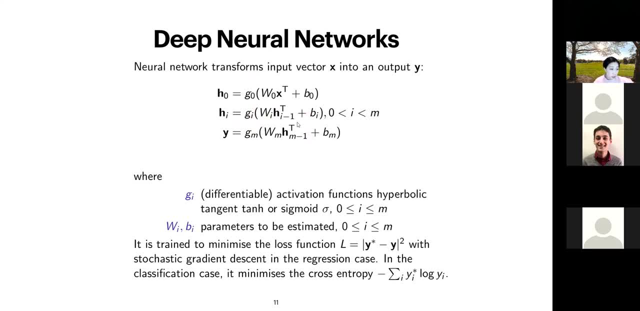 and then another activation, non-linear transformation. So you do that composition again and again. So the number of times you do that is the depth of the neural network, And then finally you look at the output. okay, So the output is also a vector. 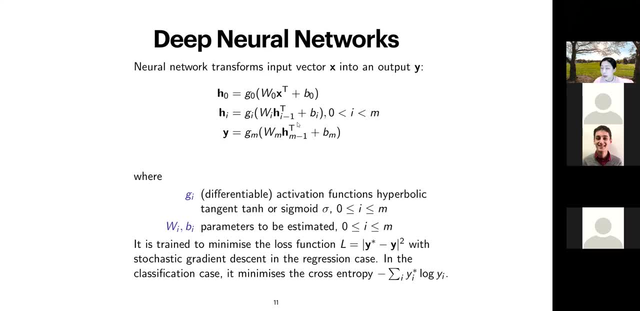 The input is on the vector. Usually input is in a very high dimensional space and output usually is in a smaller dimensional space. Okay, So this is just a very brief, I guess, recap of deep neural networks. So essentially you know, for example, 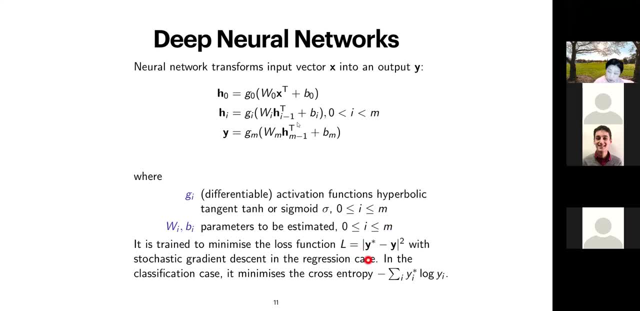 if you think about regression problems, usually you would want to reach, you know, minimize reconstruction error or kind of like. so you know some kind of- I guess it doesn't have to be this form, it doesn't have to be, like you know, the L2 norm of the differences between the vectors. 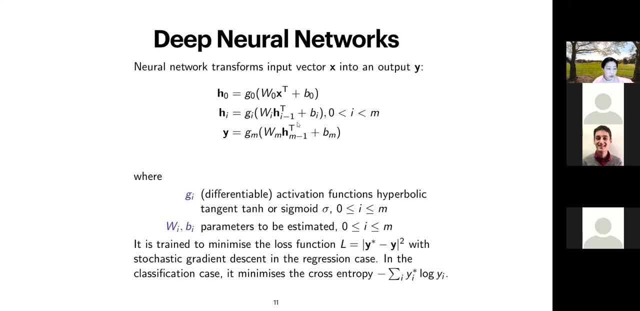 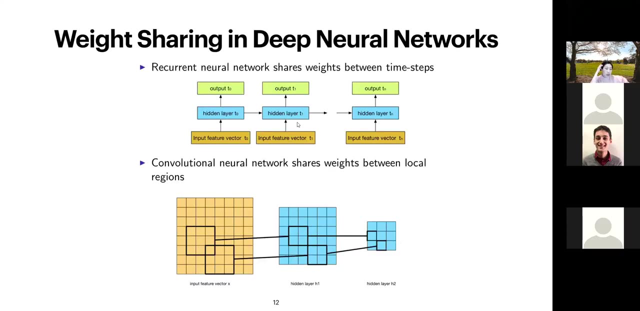 it could be other forms, but I'm just using an example here. well, if you think about classification, then the most popular loss function is the cross entropy loss, as you know we might have all be familiar with. so one important thing is, you know, in deep neural networks there are kind of weight. 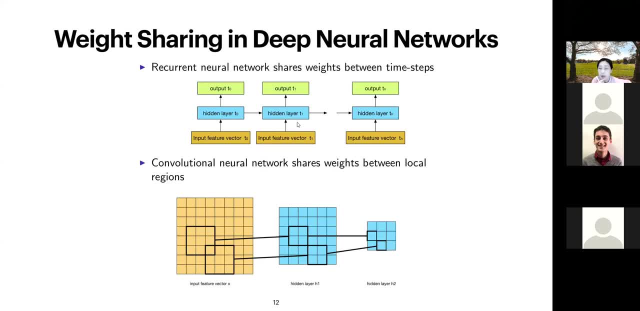 sharing, right. so? so, for example, in recurrent neural network, and you have the weight shared between time steps and you also have the weight shared in convolutional neural network, which is the more popular kind of neural networks used in you know, kind of images, or language models, or video models and so on. okay, so now, finally, you know we're here at the 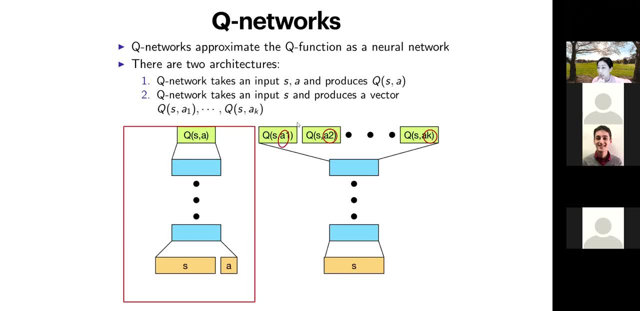 next slide and I'm going to show you how to get to the next slide. so one of the most popular non-discriminatory neural networks is called Q-networks. so Q-networks are essentially a function approximation of the Q function. so it's using a neural network. 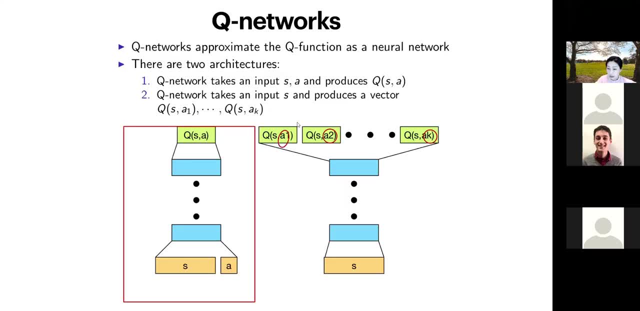 but you can imagine two ways of designing Q-networks. so here on the left hand side, on the right hand side, on the left hand side is the Q-network: take an input S and also an A. it says: take an input state and action. so you know, state and action might have been wrapped into vectors and 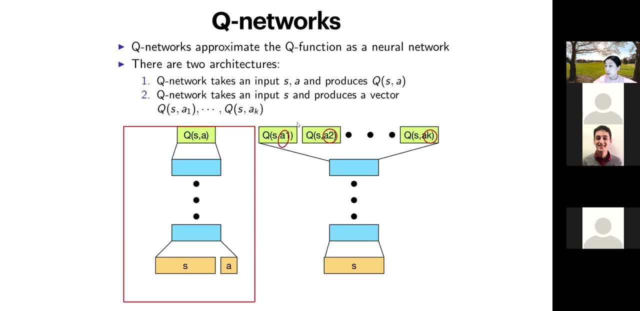 in a D dimensional space. then you produce the QSA. So this is the value conditioned on S and A. So that's one way of designing Q networks. The other way of designing Q networks, which is actually the more popular one, especially popularly used in Atari games and so on, 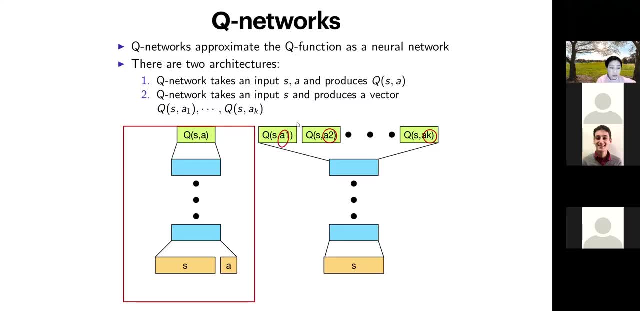 So is this on the right hand side? So, indeed, your input is not S A pair, but only the state. So it's a state where you know. back to representation of the state. It could be an image, right, It could be a video, it could be, you know. 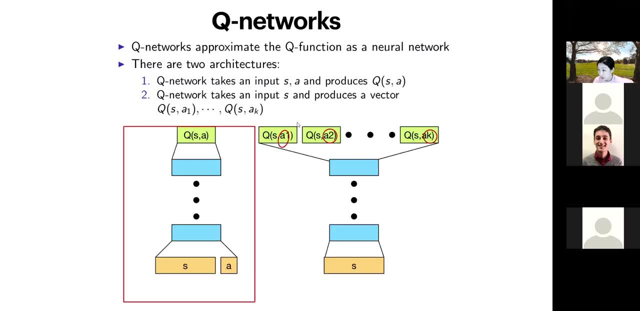 it could be, just like you know, a discrete state also, Right. so then you go through a neural network, but the output is different. It's not the Q values itself, but it's a vector of Q values. So each entry is corresponding to a different action. 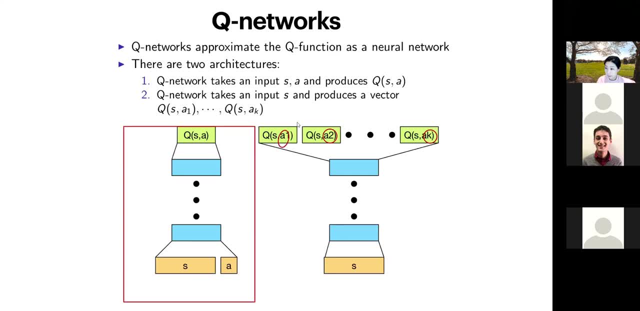 So you can imagine, this is for finite action space, right? So you can see. so, the first entry corresponding to the Q value corresponding to action one, second entry, action two, and so on. right, So all of these Q values are corresponding to the specific S that you input to the neural network. 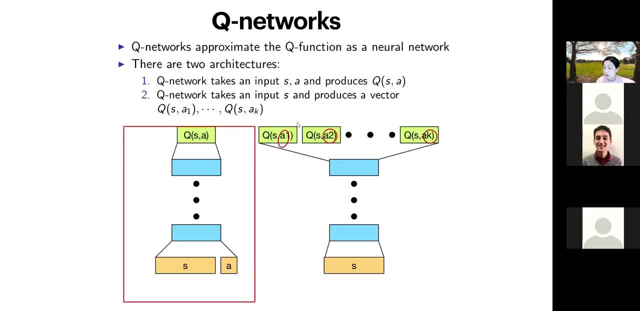 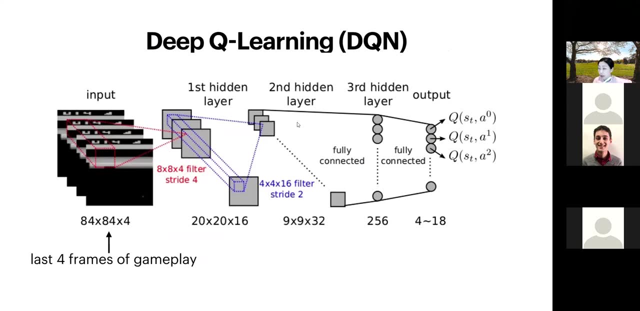 Okay. so this is just a description of the Q network And, more specifically, here is an example of the deep Q learning, so-called DQM network. So you have the last four frames of the game play as the input, okay, And then you go through a CNN, right. 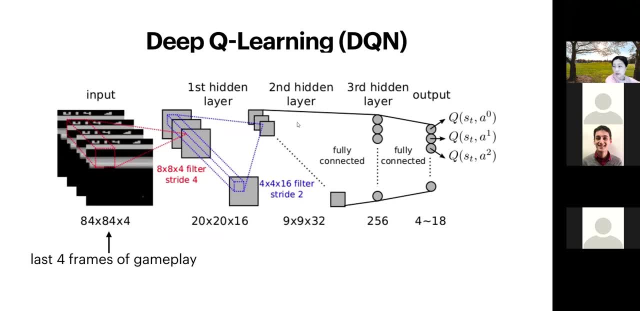 So you have like eight by eight by four filters, strike four. And then you have like four by four by 16 filter, strike two, And then you go through a fully connected neural network, actually you know. second, So you have two layers of fully connected network. 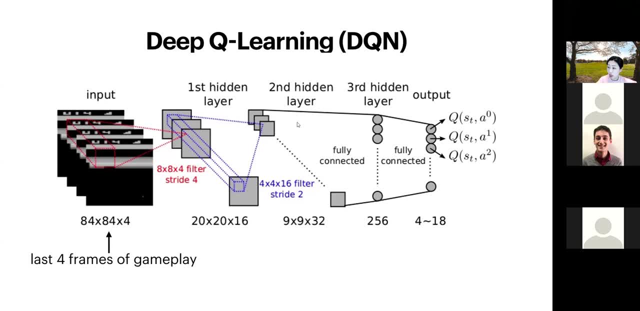 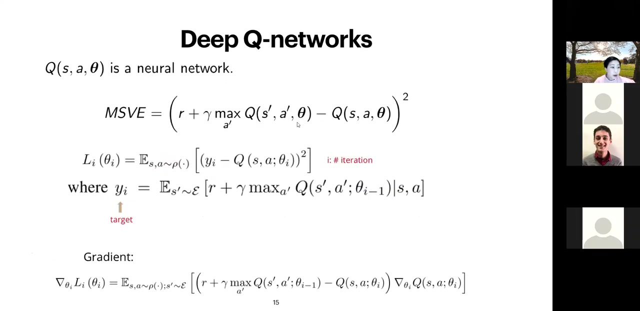 Then the output is corresponding to the vector of the Q values, each entry corresponding to one action in your action space. Okay so this is a- I believe this is, you know, a popular deep Q network used in Atari game. Okay, so now with this deep Q network, 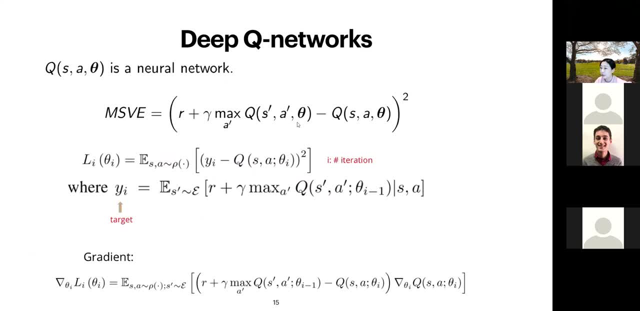 So you know you would ask me: how do I do training? So for a neural network? you know you choose a architecture Now. so it really is a matter of choosing a loss function, right? So a naive loss function is actually this so-called MSDE. 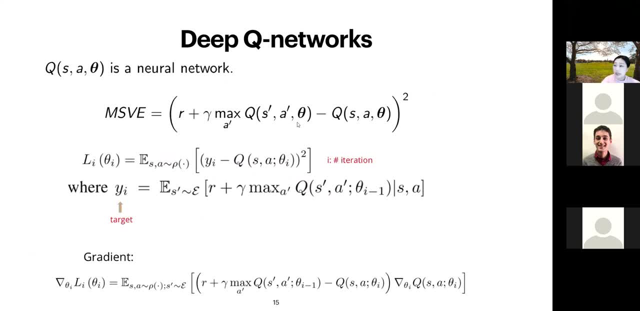 We've seen that before. So it's, you know, it's like a TD era, right? So think about the TD era. You have the R, which is the one step reward, plus the gamma of the max Q S, prime, A, prime, theta. 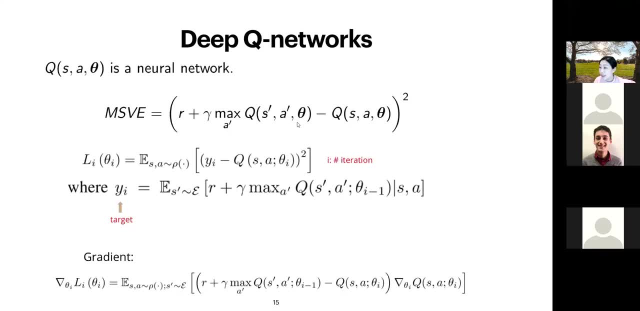 So this is very much like a Q learning essentially, So it's basically mimicking the Q learning objective, right, Although Q learning was an iterative algorithm based on TD era. here is like using this TD error squared as a objective function and do back propagation. 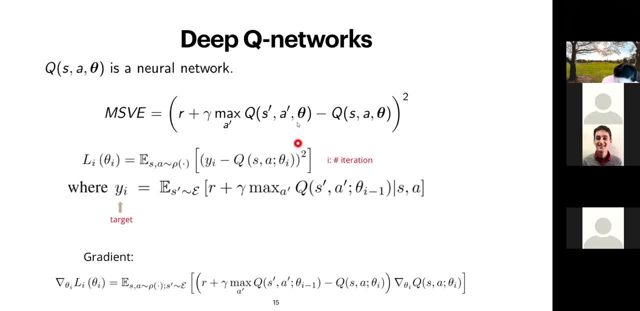 So you know, first let me see. So this is the MSDE. okay, So you can see, I have theta here. Theta, now are the parameters of this deep Q network. okay, So now I can also write it as Li theta I. 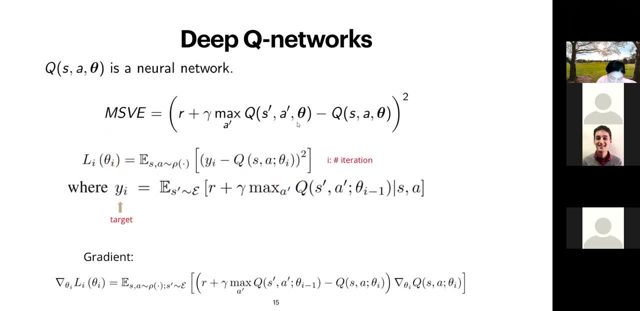 just so you know, this is my I step right So I can write this Y, this y. as you know, this part is my y, i right. so this is kind of like my target, and then this is something that's going through through my network. okay, so if you look at this, 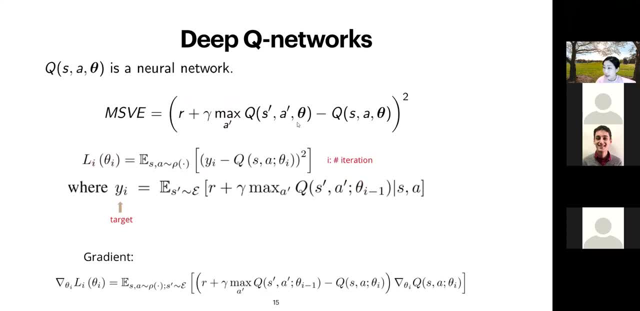 form. this is very much like what you're familiar with: a regression problem using a deep neural network, right? so you have the target and you have the input and you're finally getting the output through the of the network. you wanted to minimize the reconstruction error and, of course, 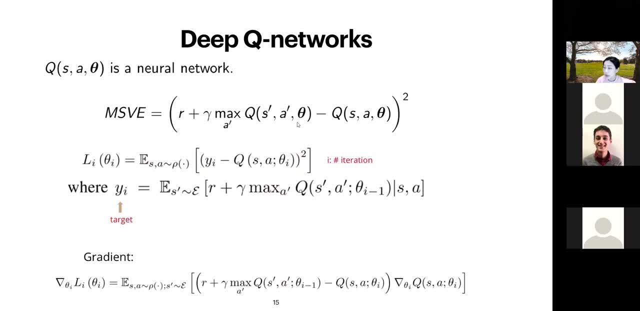 you would take an expectation over all the data examples you're looking. but one thing interesting about this is, like the data examples are no longer iid, they're actually from a- uh you know- mdp, so the trajectories are correlated with each other. okay, so, as i said here, you know. 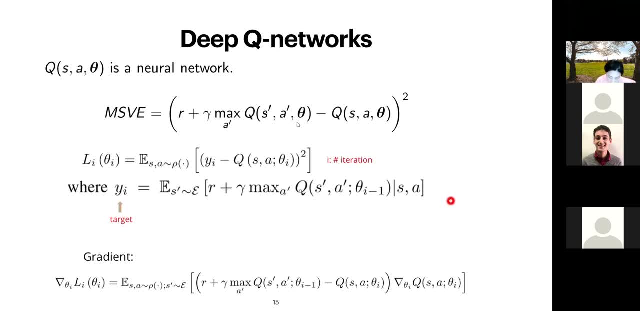 this y, i can be thought of as this guy here. okay, so now what do you do? you just take gradient, normal. you know normal thing that you will do for learning, uh, for deep learning. so you take a gradient, you get this form and essentially this is how you know deep q networks doing. 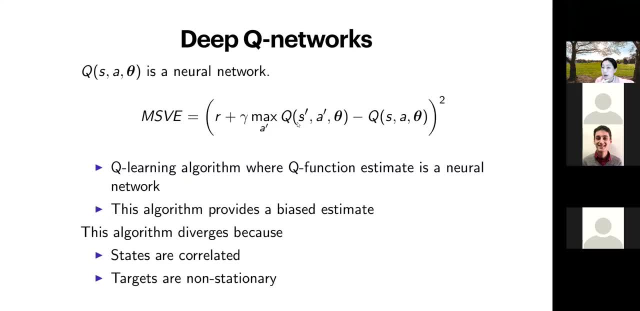 okay, so is there any problem related to it? right, all right, first of all, you know, of course, i wanted to mention that q learning algorithm is basically a q learning algorithm, but the thing is that q function estimate is actually a neural network. but the problem with this 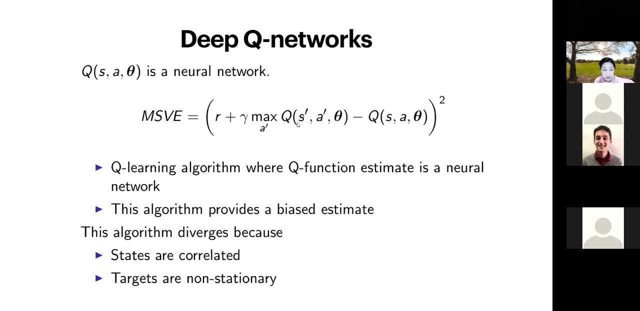 the algorithm actually provides a biased estimate and, more importantly, this algorithm could diverge because the states are actually correlated and the targets are non-station stationary, okay, so this is really problematic. so, to solve these problem, i think the you know, the most important contribution of this deep q network paper was to provide two key mechanisms to solve. 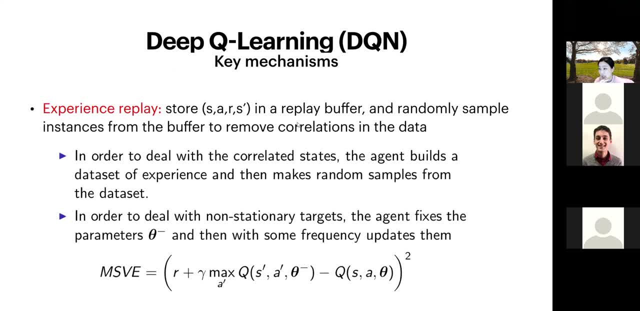 these problems. one is so-called experience replay. so what is it? so it may- it might be something that's really heuristic- to solve these problems. and the other is to solve these problems. so what is the so-called experience replay? so what is it? so it may, it might be something that's really 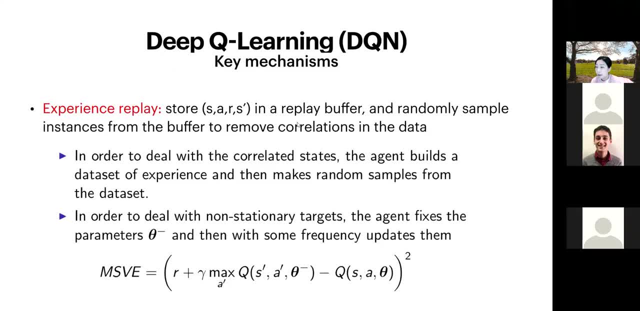 heuristic at first sight, but it has a principle consideration behind it. right? so if you store, so what is the experience replay? if you store the s a r s prime, so this tuple in the replay buffer, okay, so you do that, and then you randomly sample instances from the buffer. 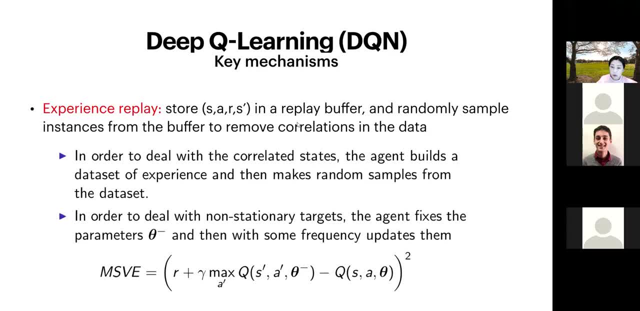 now you can see that the data is actually stored in the replay buffer. so, instead of using, you know, my s a and my next step s prime and a prime, i'm actually, you know, storing things in a replay buffer and do random sampling. therefore, i can break the correlations in the data, okay, so that's a very 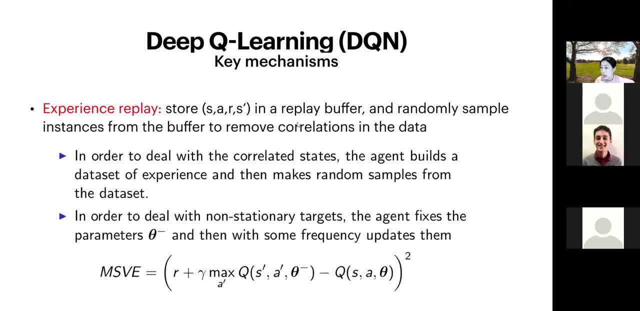 important trick that is used in reinforcement learning and, essentially, i i can imagine this being applied to many other systems as well. i can imagine this being applied to many other situations where you know data is correlated. okay, so, more specifically, in order to deal with the correlated states, 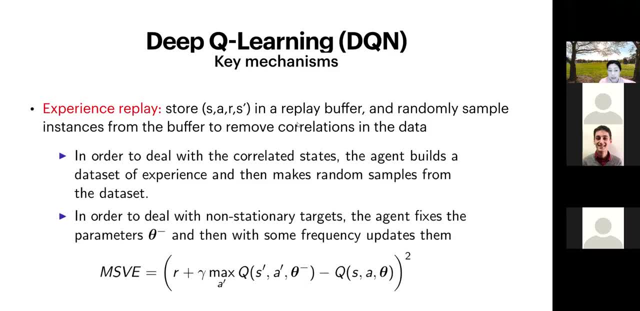 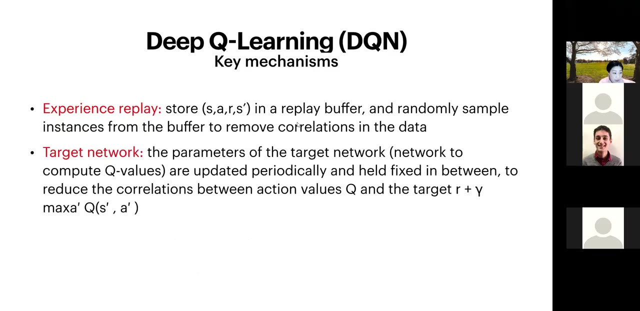 the agent builds a data set of experience and then makes random samples from the data set. okay, and in order to deal with non-stationary targets, actually the agent fixes the parameter and then with some frequency, updates. so so what does this mean? this just means a target network, so the parameters of the target. 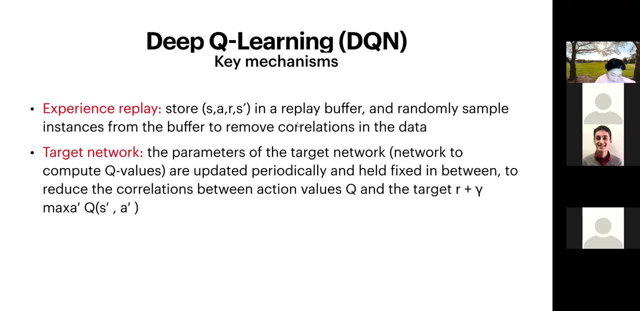 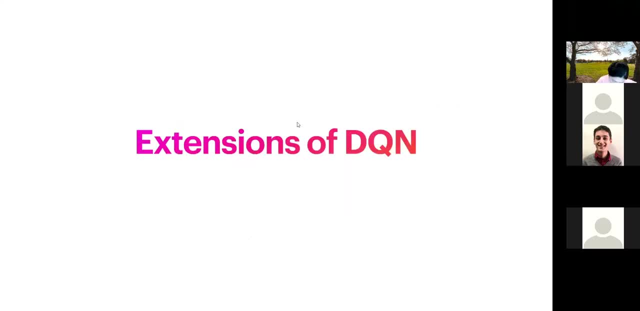 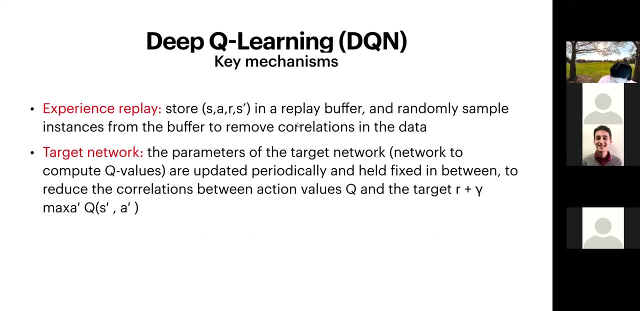 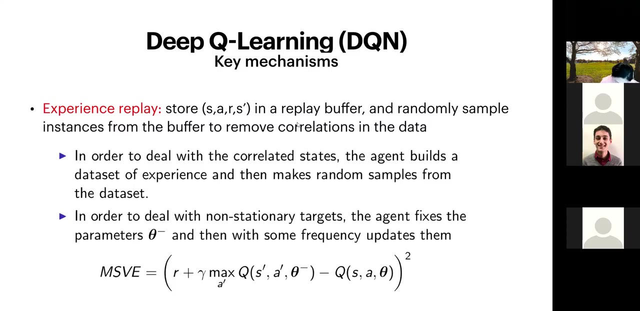 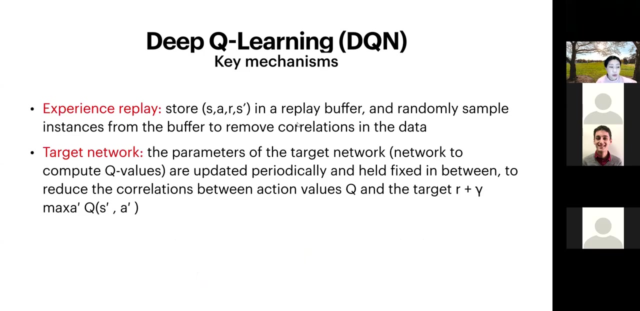 network are updated only periodically, like i said in the previous slide. oh, what happened? um here. so, in order to deal with the non-stationary targets, so they choose to update this network periodically. so what this means is that, um so so the parameters of the target network. 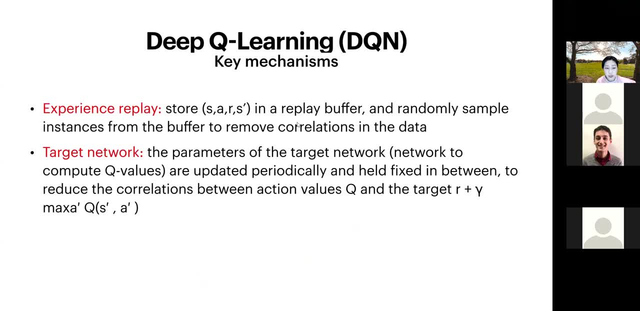 is only updated periodically and held fixed in between to reduce the correlations between action values q and the target, which is r plus gamma. maximum a prime, q s prime, a prime. okay, so basically these are the two key mechanisms for deep q networks. it is really accuta learning using a. 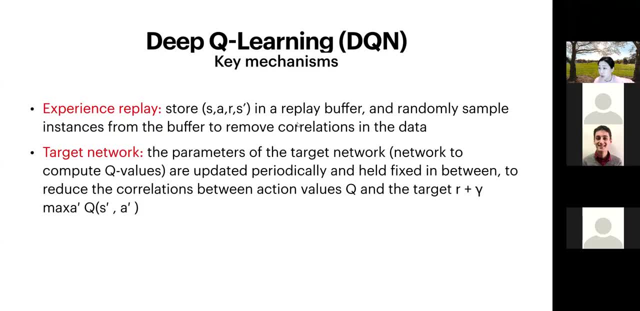 deep neural network. but because of these difficulties or challenges, um, the authors have proposed two mechanisms to deal with it: experience replay. i think it's gonna change dinner, but what neaya did is? she launched this. get back see, it is missing for one second. sometimes, very often, there is because of the Egyptian mathematicians. this established a network where the investors quite often three to four devices, such as two. 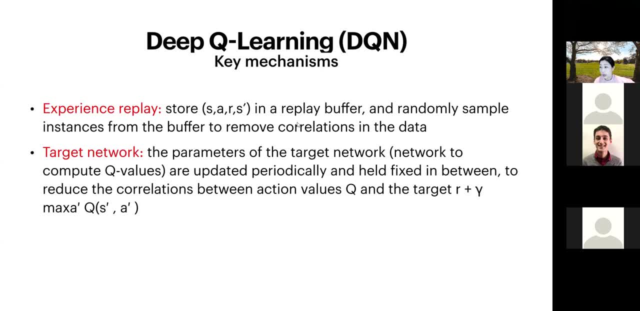 we can define the drivers in the data sets and the other risk theputyou and the- just the dobrze 我 type it- the ones with your data sets and values, q and the target, which is r plus gamma, maximo a prime, q s, prime a prime. okay, so basically these are the two key mechanisms for deep q networks. it is really accurate learning using a deep neural network, but 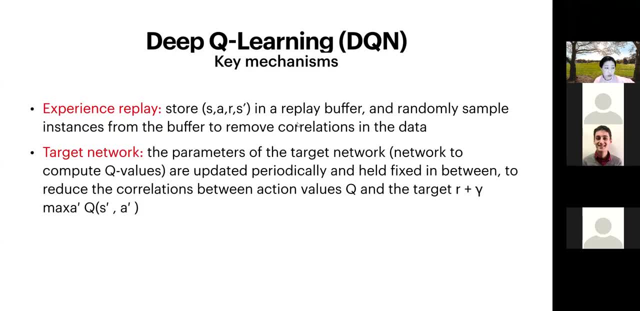 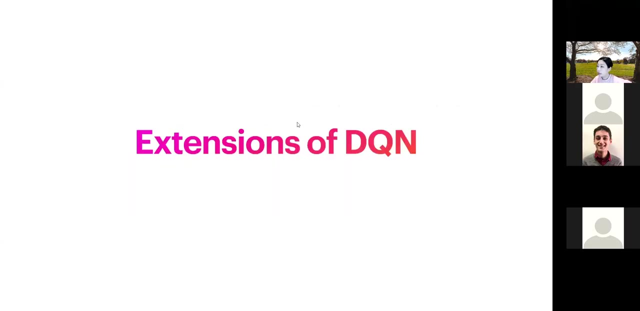 I think it's really useful for other situations as well- And the target network. I also think that this trick could be used in general deep learning methods beyond reinforcement learning. OK, So if there is no, is there any questions? No, I'll talk about the extensions of deep Q networks. 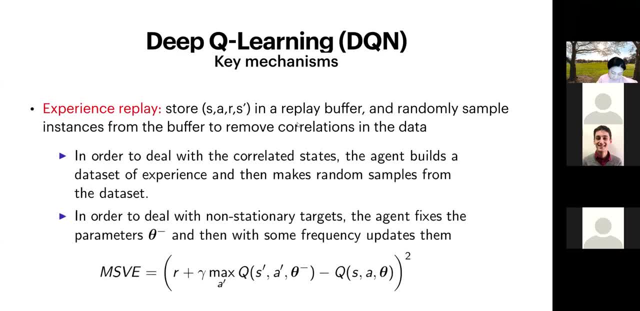 Can I explain? experience replay. You mean again: OK, So you store. So is there any Specific question? Nothing in specific, but it's like. so while training, one input sample will be one experience, or like, because each data sample is not IID. 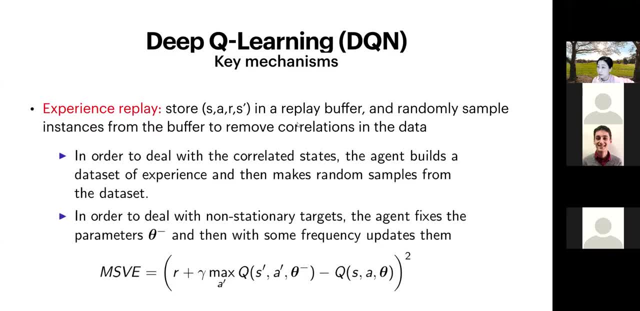 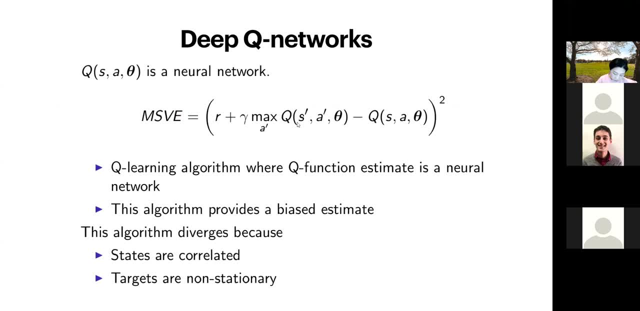 So I mean I'm not able to understand how replay is done, Right? So you wanted to use examples to minimize. So how do you estimate the function value of your object? So you use examples And the way that you're using samples. 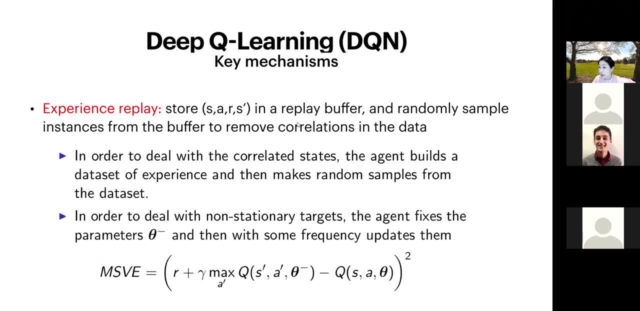 are not based on trajectory but based on a replay buffer and randomly sample from that replay buffer In Q learning. you would follow the trajectory right. You follow your implemented policy and you were collecting this epsilon-grading policy actions and rewards and transition to another state. 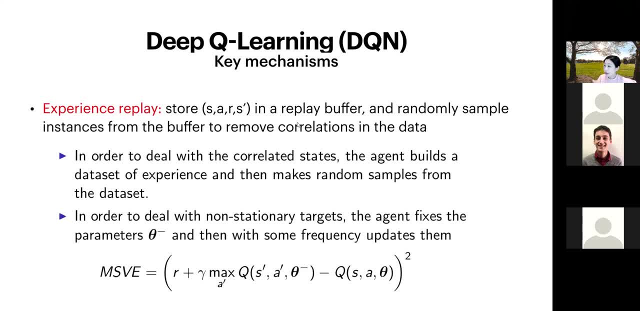 You're collecting those based on the order that they appear right. So, based on the order of the epsilon-grading policy that you're implementing Here, you might also be implementing implementing something similar, but you do not collect samples based on the order of how you. 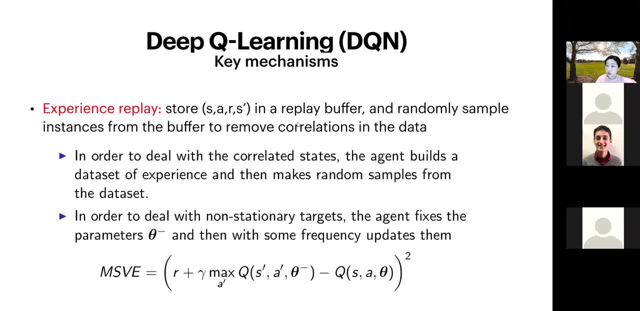 observe your triples- sorry, this is triples. so instead you would store them in a buffer and then do random sampling. so therefore, yeah, each one's, you know. so there is a high probability that you won't collect the examples in the way that they come, in the order that they come. 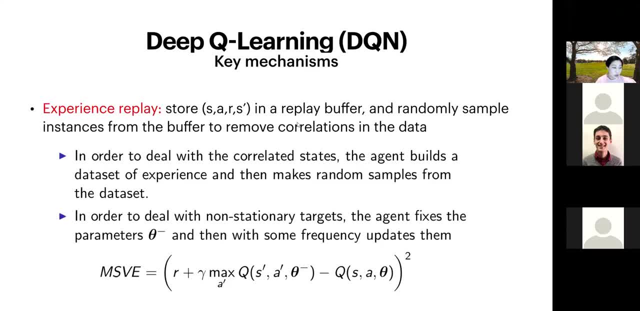 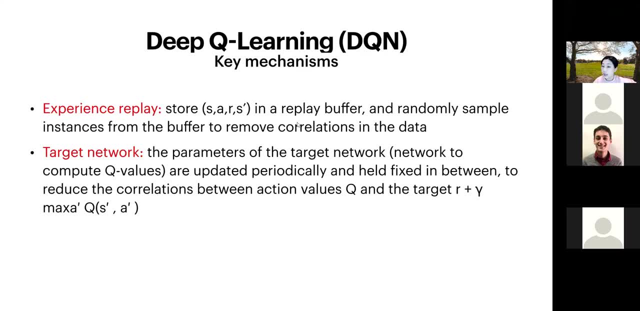 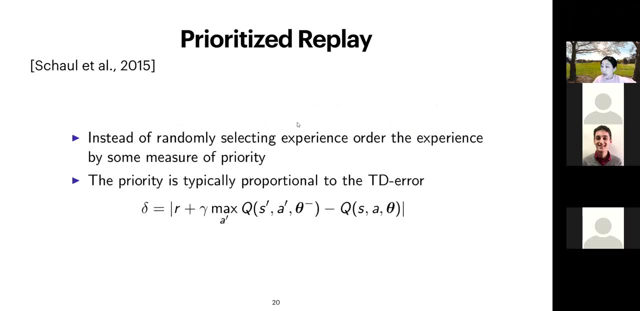 okay, i got it, thank you, yeah, sure, um right. so i guess is this clear. okay, all right, so let's see the extensions to deep q networks. so one, uh, extension of the deep q network, other than doing these two tricks: right experience, replan and target network, updating it periodically. so this is the 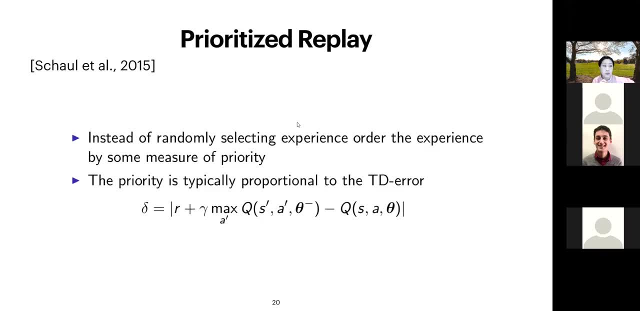 uh, first extension of the deep q network, which is the prioritized replay. so instead of so you know. just like what? um, um, sorry, uh, let me not pronounce your name incorrectly. just like what you asked earlier. um, you know, because you have the experience replay, you're sampling from the buffer, but now, instead of 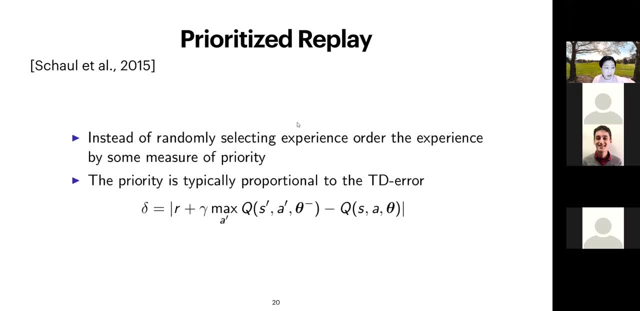 doing a random sampling with uniform weights. um, we wanted to do something with kind of some priority. what priority would make sense, right? so this prioritized replay is suggesting that you sample the examples in the replay buffer, um, you know, with a importance way that is proportional to the td error. so what does? this mean. so this basic question is like a test to see if, if we are able to make results from the beginning of a circuit where you know, if you know, the application is not going to the end of the process, so how do we do that? so there are several possible ways to actually test that. you can use the 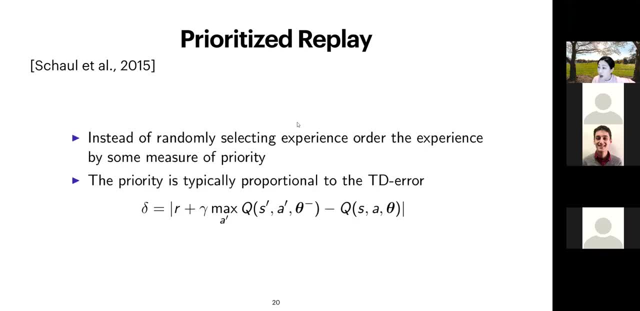 means that if the td error is large, so that means i haven't learned a lot in those state and action. right, because my values for my value estimation for that state and action is just very bad. it's not accurate. right, because you know if td, whenever td error, is close to zero, then we've 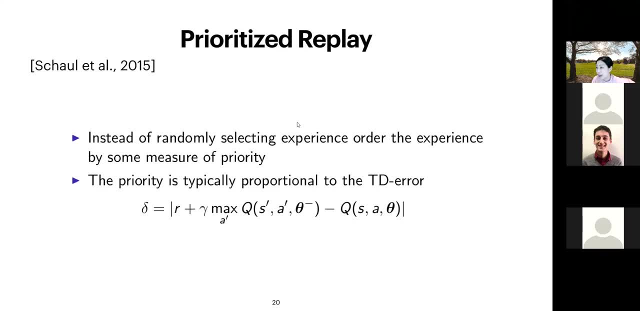 converged to some kind of optima, or either local or global, but some kind of optima, but here the td error is large, then that means we still need to do a lot of work in estimating the state and action values. so it makes a lot of sense to sample the data that has a higher td error. 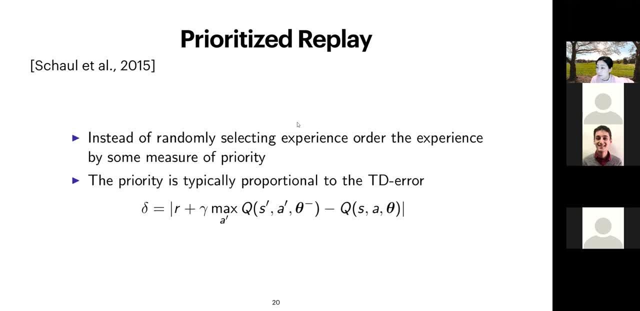 with higher probability. okay, so then the importance weight is really just something that's so. the design is to have the importance weight of sampling proportional to the td error, and that's a very simple idea, but it worked very well, although i don't have, you know, the. i guess i didn't put the results here, but so you. 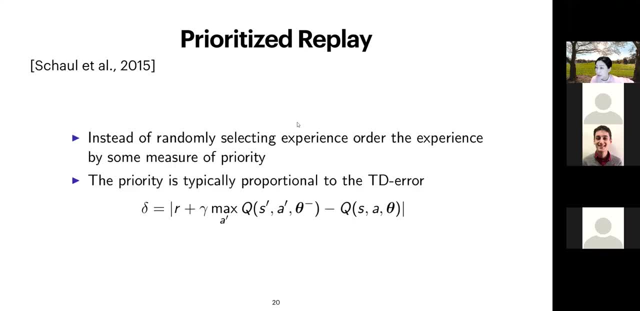 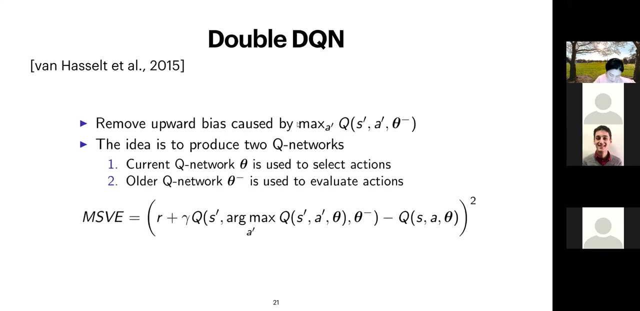 can take a look at the paper. um, indeed, it can achieve some kind of improvement. okay, so the, the, the, the. this is one extension of the deep q network. any questions so far? okay, now i'll go to the next one. so the next one is the double dqn. so double dqn. 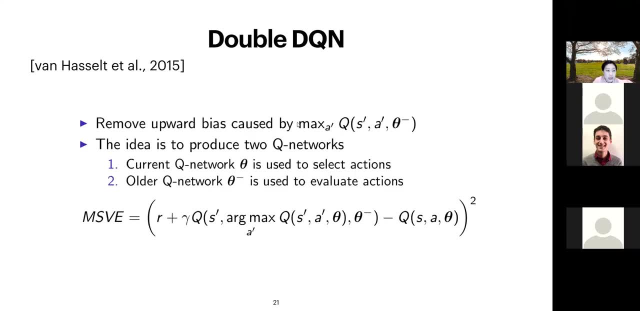 also proposed in 2015, is to remove this upward bias caused by the maximum of the q s prime: a prime. so the next one is the double dqn. so the double dqn, also proposed in 2015, is to remove this upward bias caused by the maximum of the q s prime: a prime. 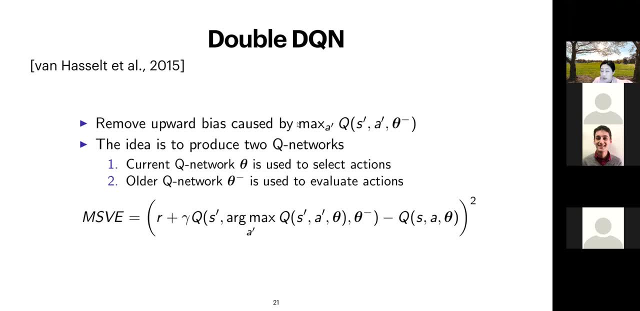 so the next one is the double dqn. so the next one is the double dqn, so the maximum of the q s prime a prime theta minus. so the theta minus is causing some kind of bias. the idea is to produce two q networks before we only have one q network. 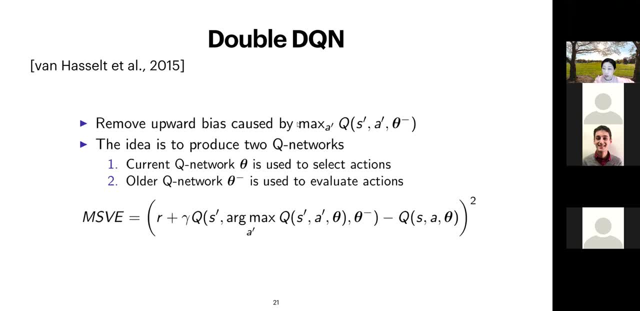 now you can have two q networks, is you know, one is the current q network, the other is the older q network, so it's like a delayed copy of the current q network. um, so in the current q network you're going to use that for selecting actions, right? so because you know you wanted to do um. 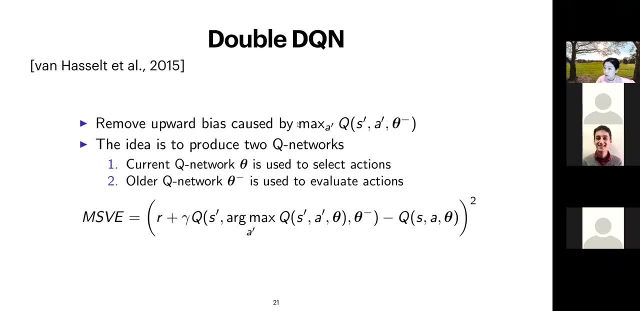 you wanted to improve, uh, the q value based on. you wanted to improve your policy, you know, based on the current estimation of the q. so you wanted to use the current q network, which is parameterized by theta, to select the action to improve your policy. however, um, you're not going to use the 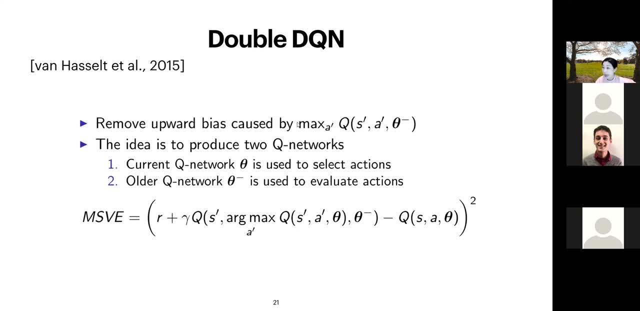 current network to evaluate these actions. what you do is you're going to use the older network, which is theta minus uh, to evaluate actions. so you can see this. so the objective function actually becomes this one. so one thing you notice is that: so here you have this q s prime, a prime, you know. 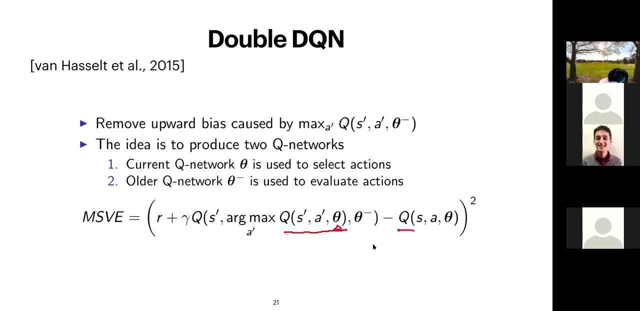 theta. so this is still theta and also this one still theta. however, uh, you have this q of s a and theta minus, right? so this is q s prime a theta. let me just say q star, because this is argmax, so it's q prime star, kind of so, however, you are going to use a older q. 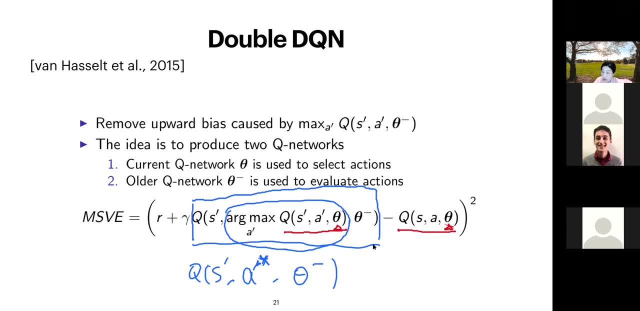 network. let's see another example. all right, that's q i who uses this q network. okay, now what is it through 36 rogue method? so this is the visuals where you have this huge cross plane, mu, and q star. will predict entry here. will predict entry here. so start with, we bring up this function to 9.1. so this is the, this: this is the interval of Sat no to 5. s is the unit of grado and so recognizing out during 18 battle times that d. so you said you can leave them up to 58 variables because you learned. 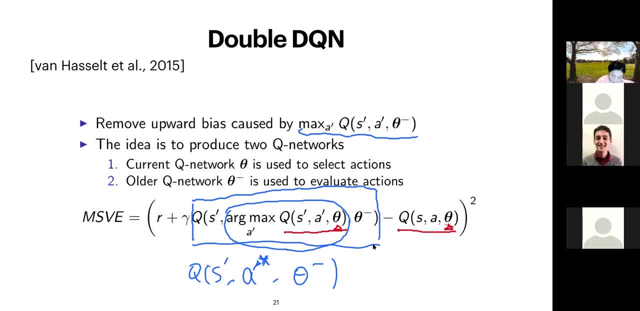 right and we are going to generate, by using that, the distance from where x wouldник, so you can媽. so the distance from right, First use this. whatever I used, you know, I marked with red So this Q network parameterized by theta. 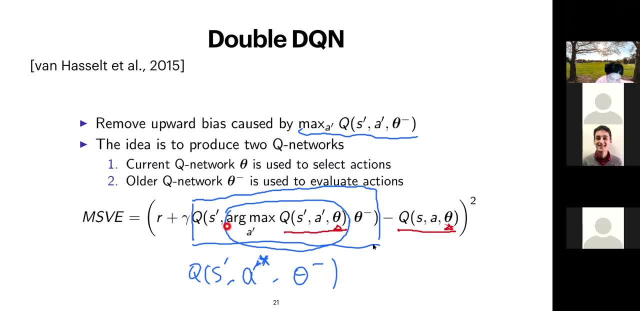 is going to use for select action, right. So this is selecting the action is argmax of this Q, but in evaluating it and then evaluating your TD error and essentially your objective, you're going to use this guy here with parameterized by theta minus. 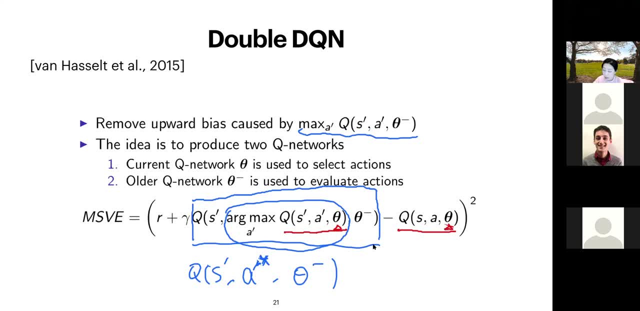 Okay, So this again seems to be a simple trick, but it solved the problem of you know. it basically is able to remove the upward bias caused by this action selection term using the same network, right, Which is you know, if you before we're using the theta. 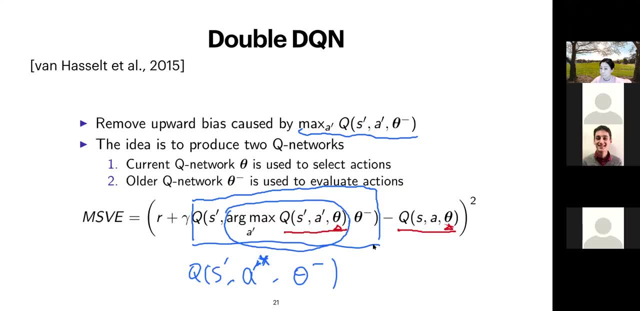 but now you're using theta minus. Is this fine? David is smiling. That's an up arrow. Joy asked the question and I am seconding that question. We're all confused by upward bias. Oh, can you explain upward bias? Oh, okay. 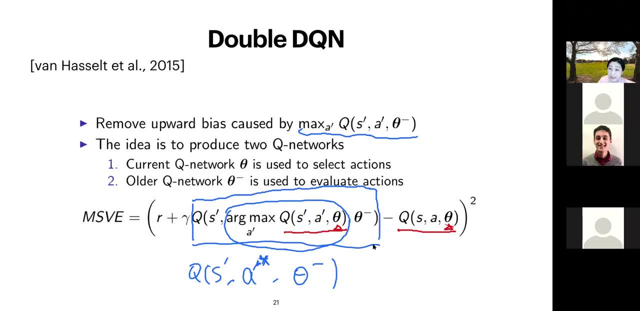 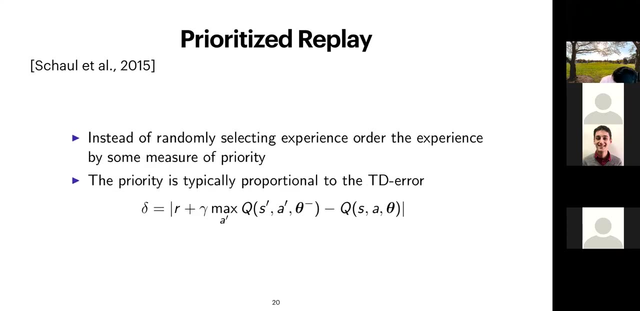 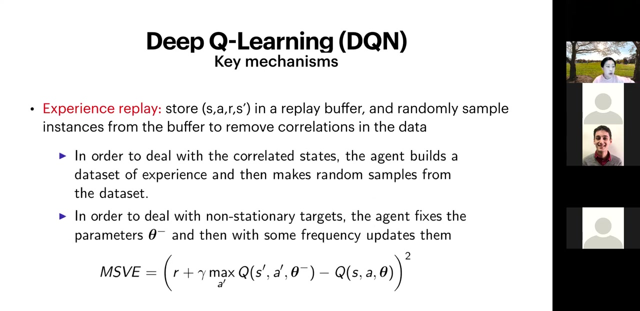 Yeah, So I didn't see that. Okay, I thought that that that was the question of explain uh, experience replay. Okay, So let me, let me see. So let's go back. Yeah, So remember, um, in the second you know mechanism, we for deep Q learning. 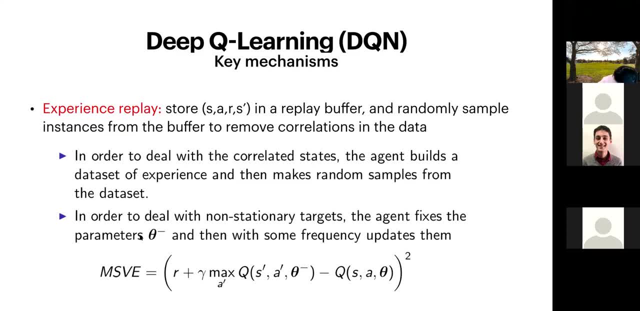 So this is the one. Okay, Let me circle it, Let me put a box on it. Can you see that? So here, what we're doing is our objective function. you know, in order to break the correlation, uh, we say, instead of using theta, we're going to use theta minus and this theta. 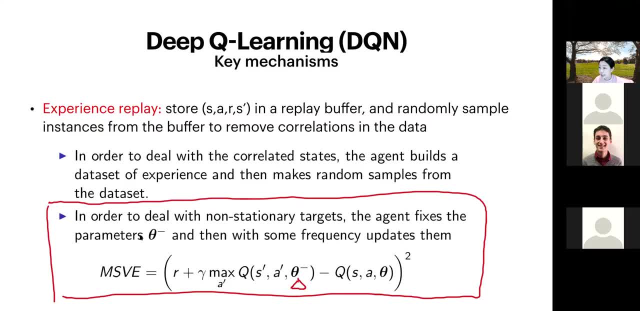 minus. So basically, you're using theta minus for selection of the action, right, Because you know our this is not our max, but max of the Q S prime, a prime theta minus. This is how you're selecting the action. 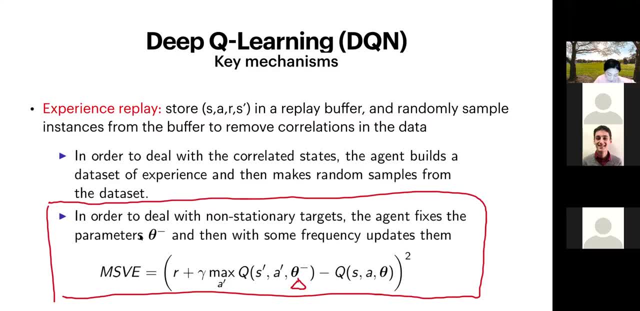 What is wrong here? you're using the one that is updated periodically, So there should be a delay in your estimation. It might be some kind of old estimation, right? We did this only because we wanted to break the correlation between the data. 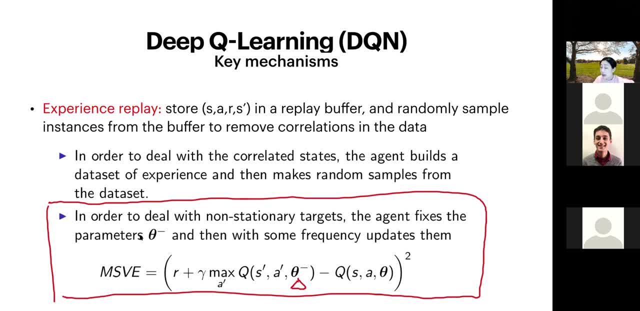 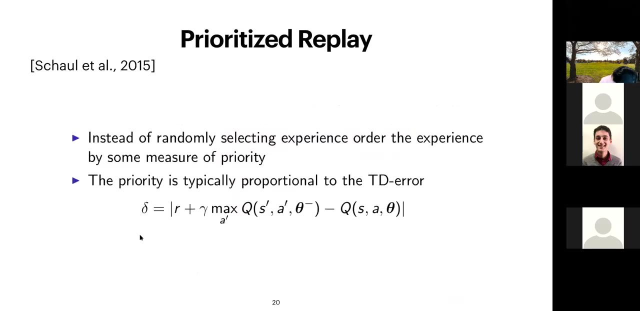 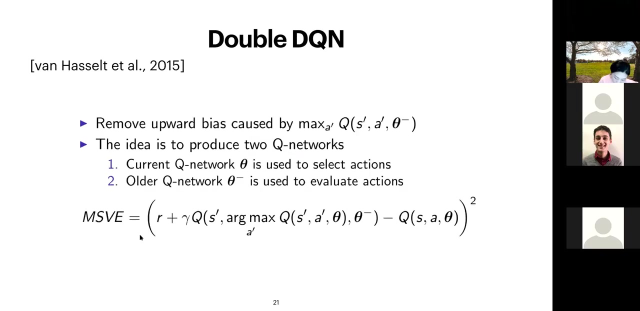 So there should be a bias, because the theta minus is not The current estimation data. Okay, So now if you see what we are doing here, Right, So the prioritized replay here you can also notice that this is a theta minus, not theta. So now if you see, oh sorry, 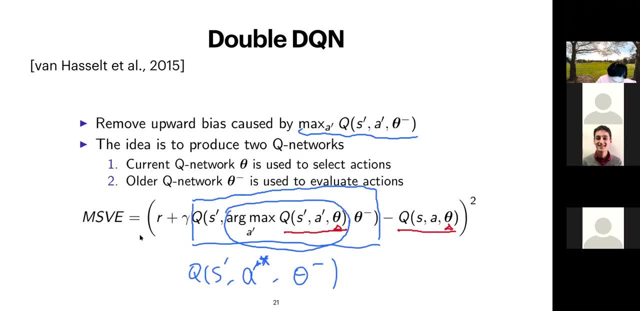 Here, Right? So if you see this slide, Uh, you can see, you know, instead of um. so so the way that I'm selecting, so before it was just like um, how should I say Yeah, So before it was. so let me put it this way: 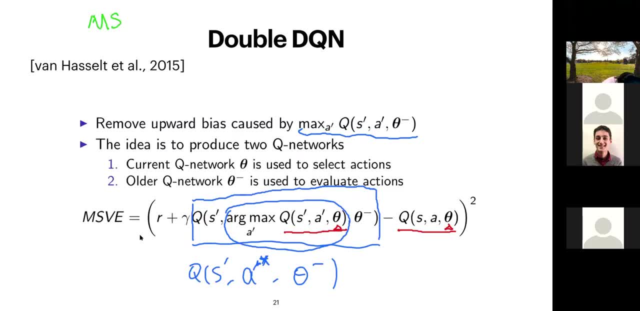 Okay, It was S V E equals r plus gamma Max a prime Q S v e a prime q s prime a prime theta minus minus q s a theta, right? can you see that? um, am I doing some thing wrong? uh, I cannot write, so I, I don't. I don't have space for the squared. 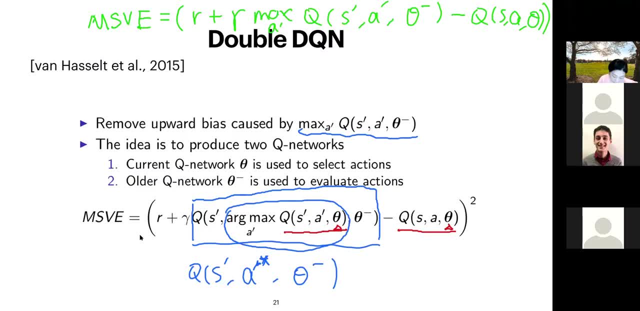 um, but just pretend that I have a squared there. okay, so this is what we were using before, but now, in this double dqn, can you see the difference? yeah, what is the difference here? right, so before you were choosing the action based on theta minus, but now you're not doing that. 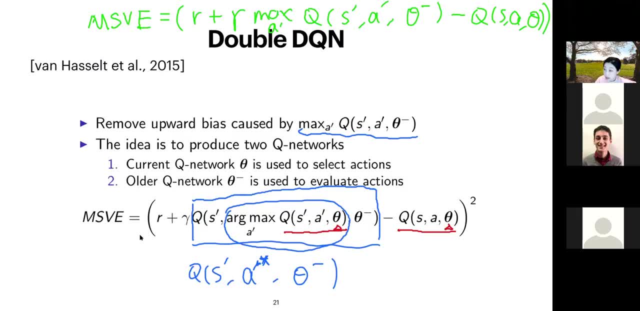 you're still choosing the action using the theta. okay, so now you're choosing the action using the theta minus, but only when you are evaluating it. you're using theta minus, do you see? uh, so I think joy is fine with it, David, do you? um? do you agree? 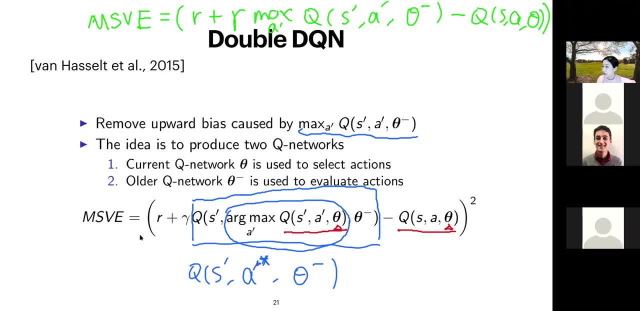 yeah, yeah, I see the difference. uh, yeah. so the difference is really. like you know, before you were using theta minus for both the selection of the action and the evaluation, but now you wanted to not use theta minus to select action. you wanted to use the theta to select action and you want to use theta minus to do. 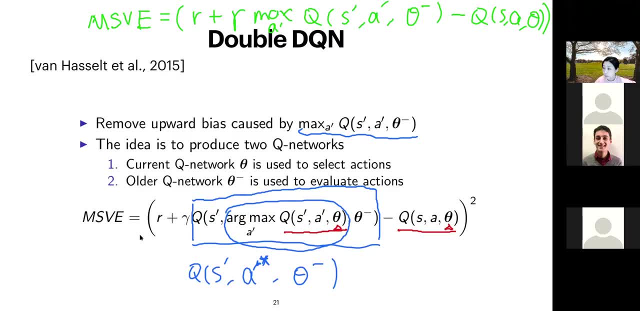 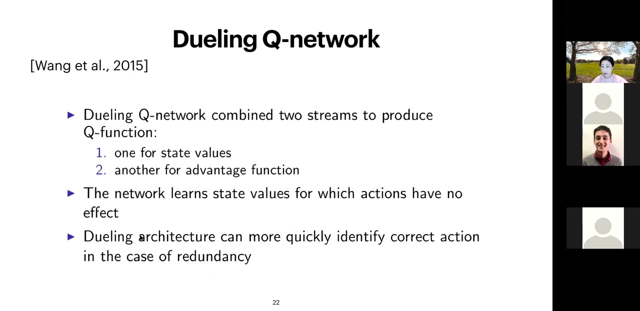 the evaluation again. so i have to say this is very empirical kind of a trick. okay, so yet there is another extension that i wanted to discuss, which is the dueling q network. so dueling q network is just another again, yet another way of doing the extension through an empirical kind of technique, which is to combine two strings. 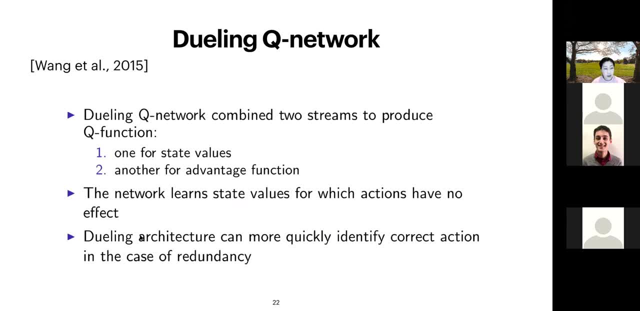 and then you can do the extension through an empirical kind of technique to produce q function. so so one is to use the state values, the other is to use advantage function. actually, in next slide i'll show you some kind of motivation why we do this. so this way then, 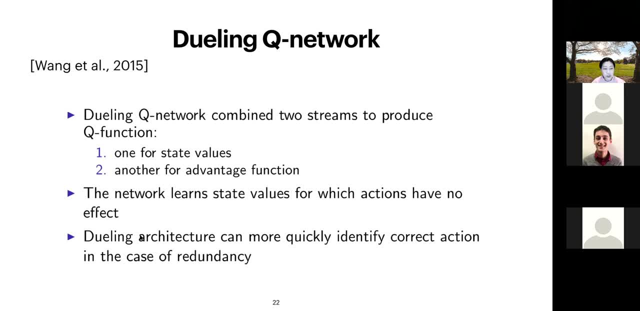 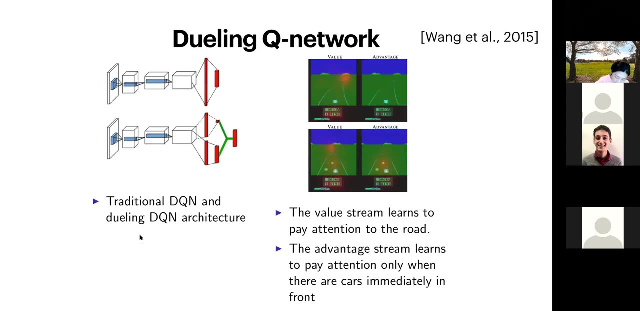 the network learns the state values for which actions have no effect. also, the dueling architecture can more quickly identify correct action in the case of redundancy. So you can see this example here. Actually, on the left-hand side you'll see this so-called traditional deep Q network and the dueling Q network, deep Q network, So that the 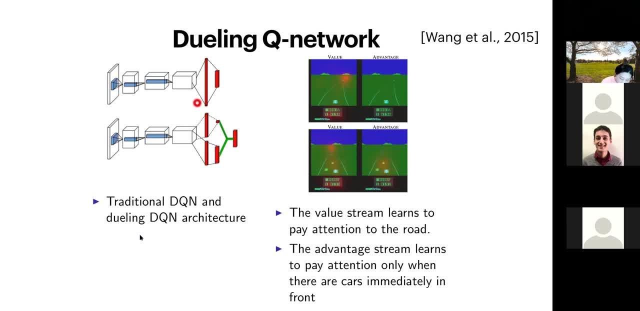 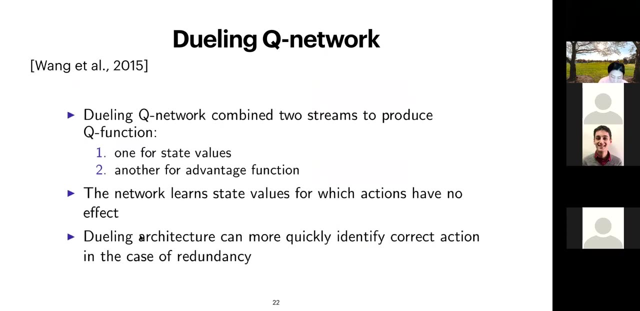 upper one here is the traditional one and this is the dueling one. The traditional one is using the Q network. So the traditional one was: you only have like the Q network. but the dueling one is combining two streams to produce the Q network. One is for state value and the other is for 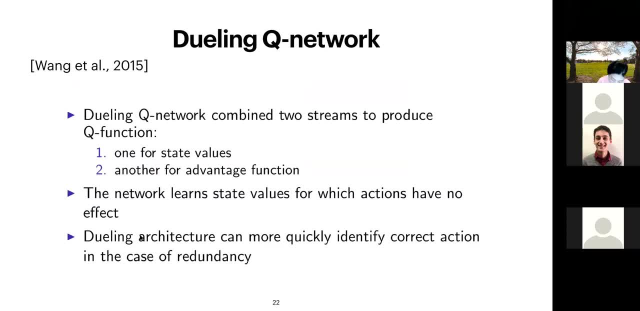 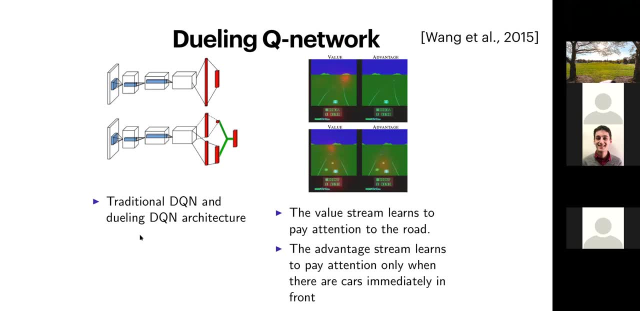 advantage function. So then the example is showing here that they have. you can see, this is a value and this is fn. So what they were saying is: the value stream learns to pay attention to the road, whereas the advantage stream learns to pay attention only when there are cars immediately in front. So, based on 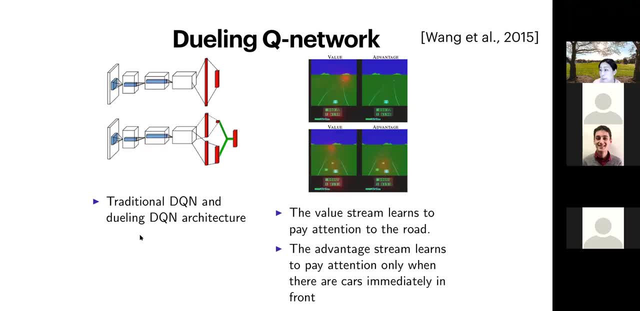 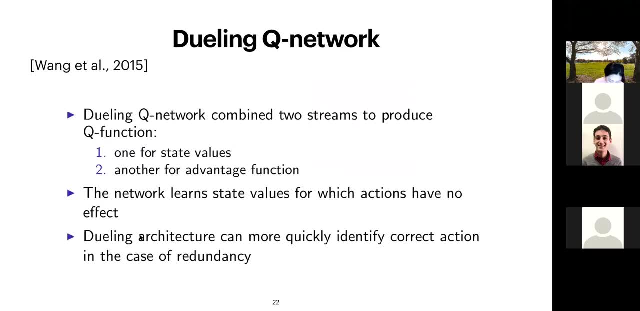 this kind of observation. they say: you know, can we combine both for the learning? Therefore you have two streams, like we're saying here, you would have two streams to produce the Q function. So they're actually really good at this kind of observation. 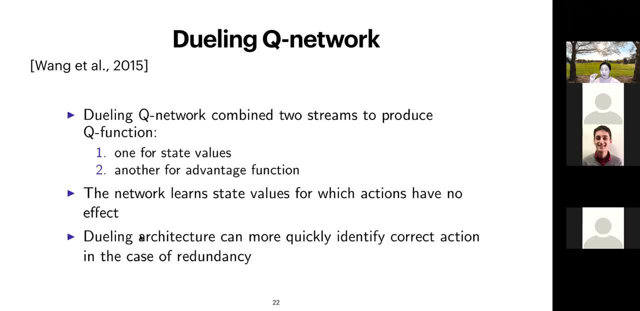 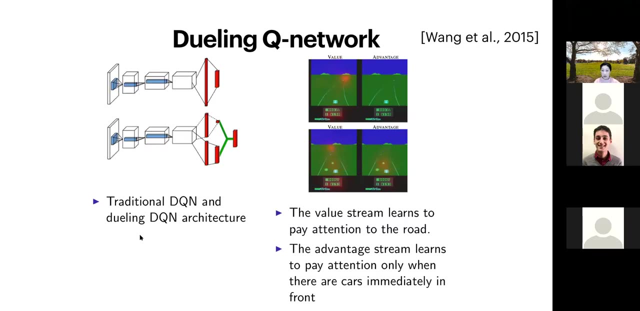 So actually I'm not really understanding the principle of this, other than this empirical observation they see in this specific game design or, you know, game design of RL agent. Okay, I don't know if any of you are working on this so you might provide some more insight about it. 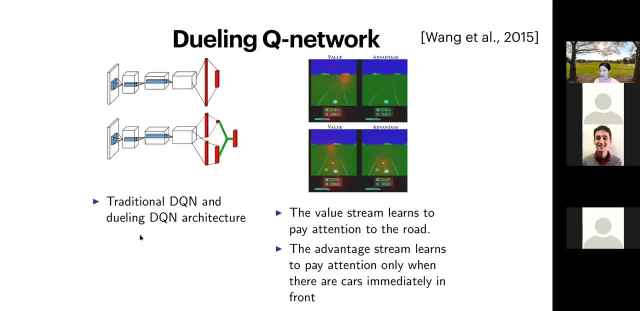 I have to admit that I'm not. my research is not on, like you know, deep Q, deep RL. Any comments on it? Okay, Is this model like multitask? I don't think so. I think this is more, like, you know, combining. 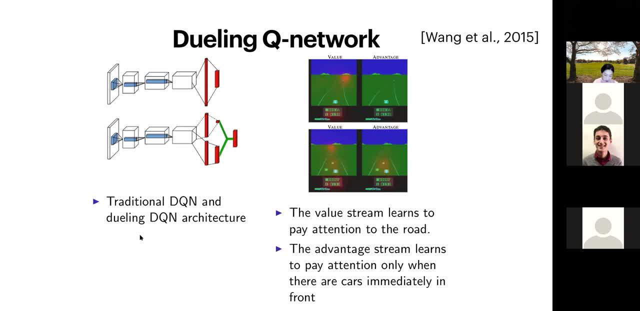 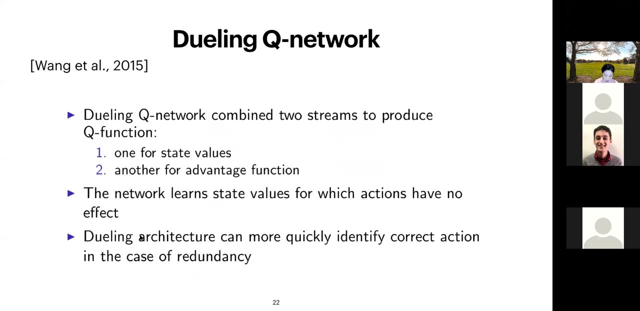 I think it's a specific design of the how to say so. you know, I don't think it's multitask, I don't see like multiple tasks involved here, but I think it's kind of like: yeah, it's like combining input, I think. 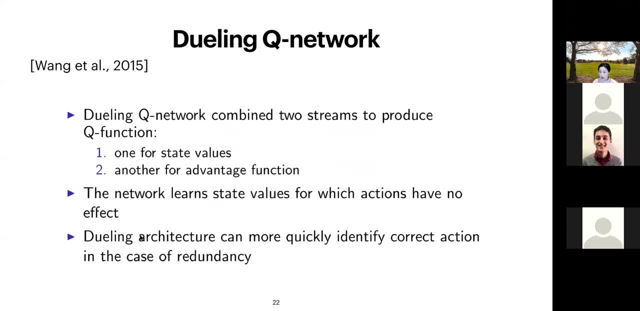 So because before your input is always like the state values, but now you have advantage function, So it's like: yeah, I don't think it's related to multitask. Okay, All these deep RL papers are extremely hard to reproduce. Well, I. 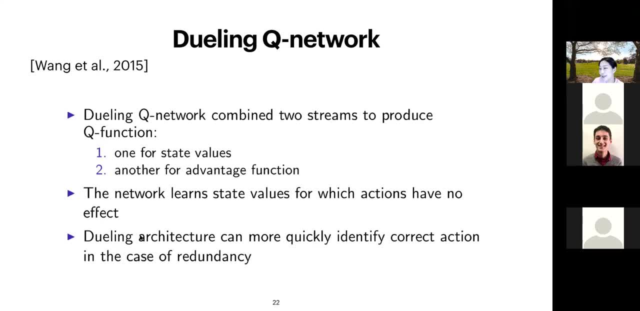 I think deep learning papers also need some kind of not deep RL also, even just deep learning papers. we need to set up higher bars for ensuring reproducibility Right, So a lot of papers. I understand that learning experiments, running these experiments, will require a lot of time. 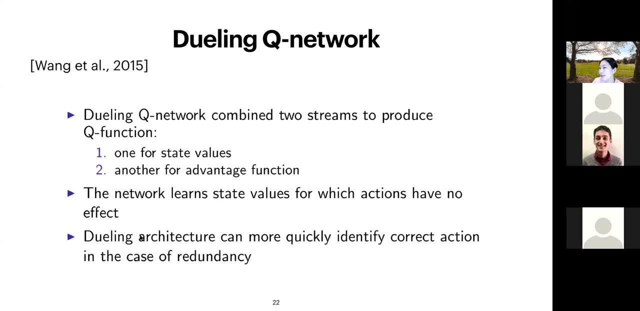 So a lot of papers do not have error bars, not have confidence intervals. Therefore, due to the randomness of the algorithm, it's pretty hard to reproduce. I agree, I haven't personally worked on deep RL algorithms. The only algorithm I worked on is a poisoning RL algorithm. 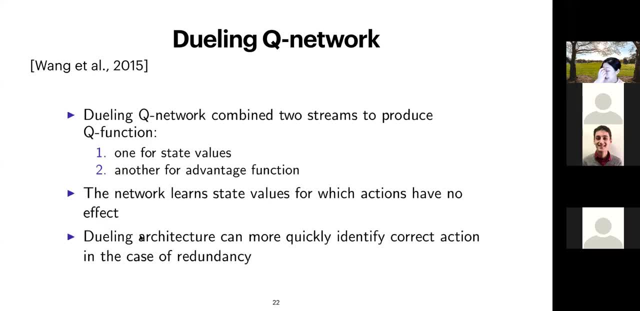 which is using a deep neural network, but I guess there isn't a lot of previous work on that. So, yeah, I guess Michael's experience is that they're very hard. So yeah, I guess Michael's experience is that they're very hard. 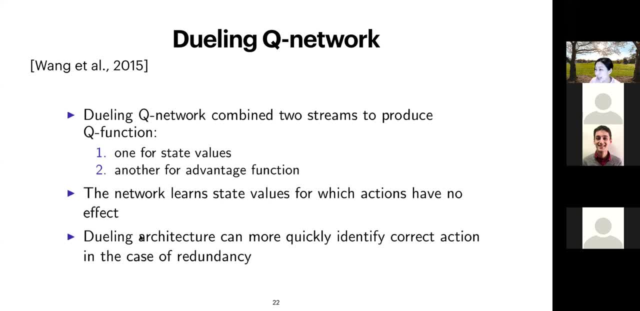 Right To reproduce. What can we do? Right, I guess we have to write in our: when we write those papers, we should, you know, make sure that we're wrong. multiple rounds with random Cs and report the confidence interval. 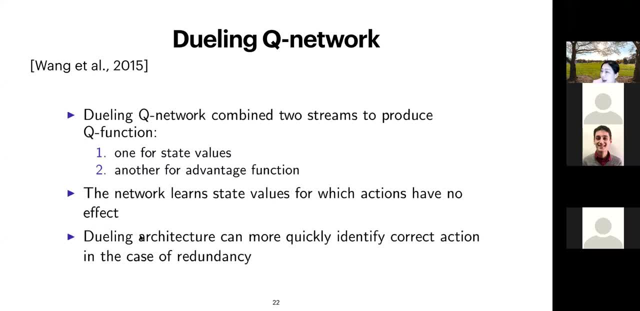 Right, So hopefully we should also, if possible, open source your code. you know, before you upload it, call: make sure it runs, set up the environment, environment using Docker, these kind of container, to make sure that the running is easy to follow. 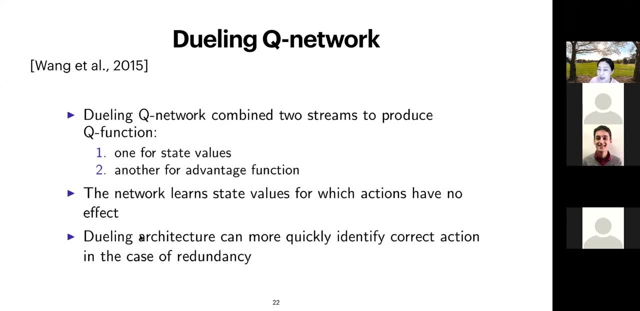 So Kyle is saying there are some githubs that implement a lot of dvrl networks. Yeah, I believe so. So so so, Michael, you know, I guess I do think that, yeah, I'm not sure if those paper, if these github repositories would help, you know, getting more confident results about these deep learning algorithms. 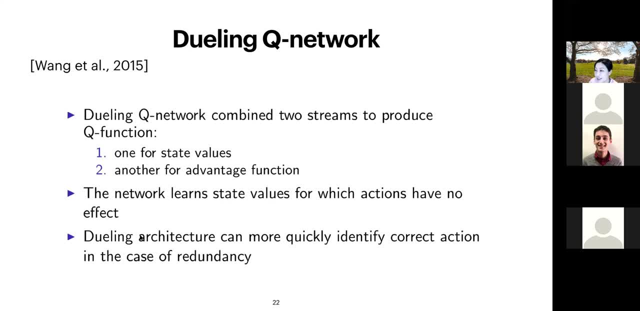 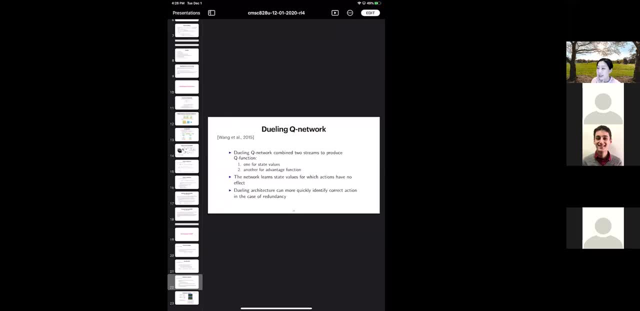 Open AI baseline. Cool, Good to know. So I can either have a. we can either have a discussion or we can continue to the next set of slides. What do we, what should we do today? We do have a few more minutes. 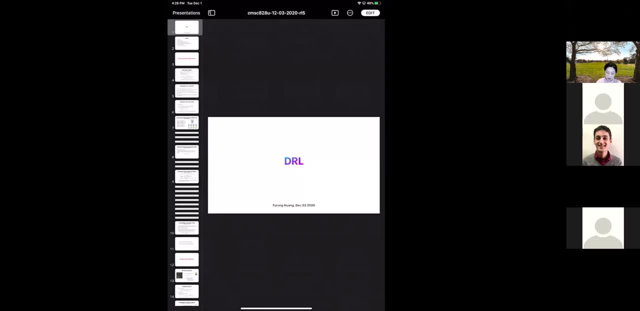 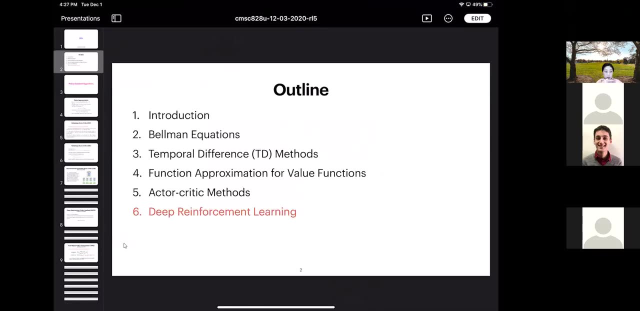 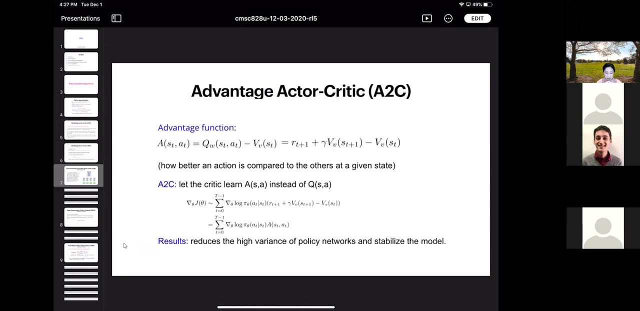 Maybe let me just very briefly introduce what I'll be doing for next lecture. So I will. I will talk about some policy gradient algorithms in deep reinforcement learning. you know, I'll talk about Advantage actor critic A2C and asynchronous advantage actor critic A3C. 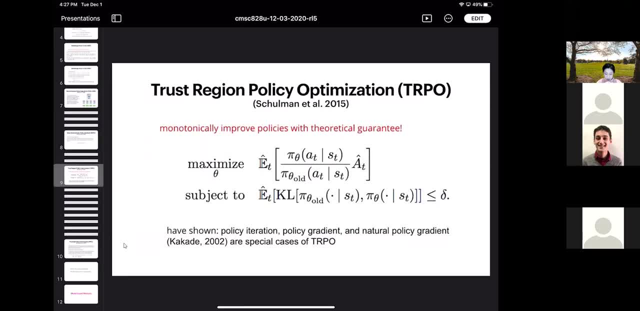 And then I'll talk a little bit more about DDP, DDP, gene and TRPO, But unfortunately I won't have a lot of time to talking about the details. especially for trust region policy optimization, It has a very nice theoretical guarantee. 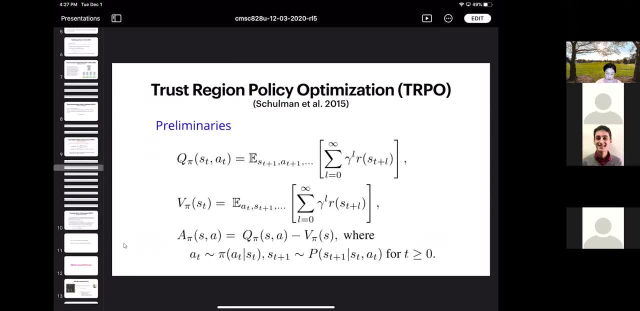 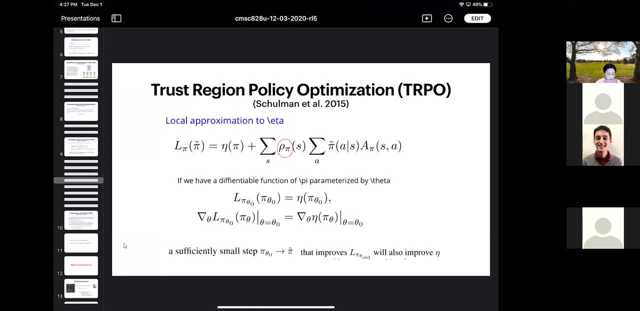 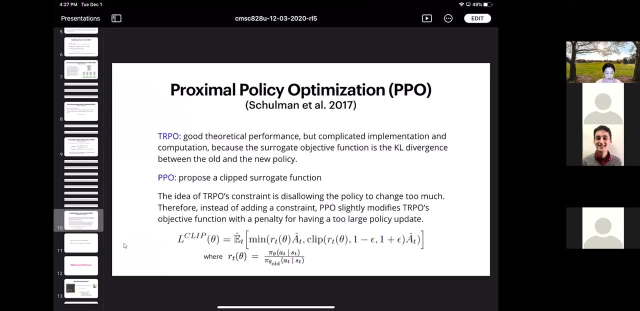 I do have some slides, but I don't. I don't plan to cover these theoretical guarantees here. I could try to share them in the slide deck Afterwards. we'll also talk about that PPO. So these are the examples of the policy based deep reinforcement learning methods.